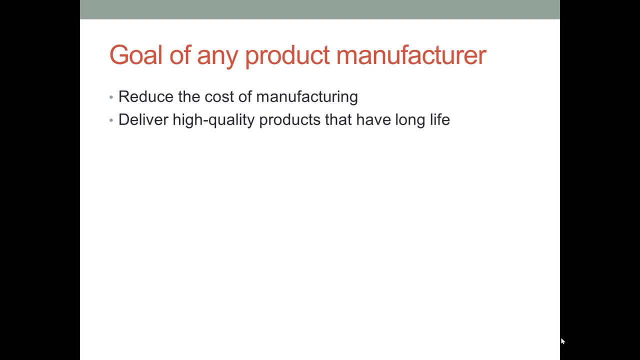 So these are the goals of any product manufacturer. So there are two or three important keywords here. One is quality and the other is, you know, long life. So we refer to them in the industry as quality. So what is quality? If I buy a product today in the market and I take it home, and if it works, that's great, you know, whereas sometimes you know what can happen is because of whatever reason right, there is some sort of a defect in the product that has been sold to me. and whenever there is a defective part, 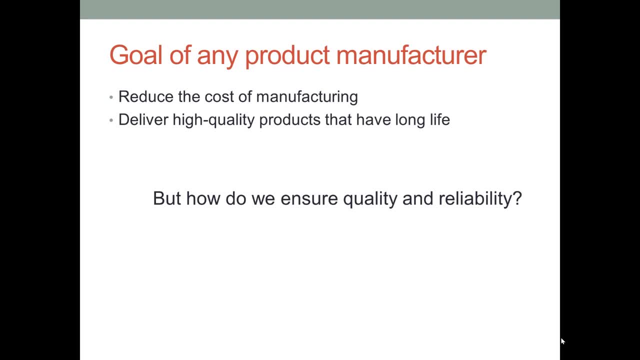 you know it is a negative for the supplier right. So usually a supplier can supply a certain number of defective parts. Usually semiconductors are purchased in very large numbers. So if I, let us say, sell 1 million ICs to a customer and out of them 100 turn out to be defective, 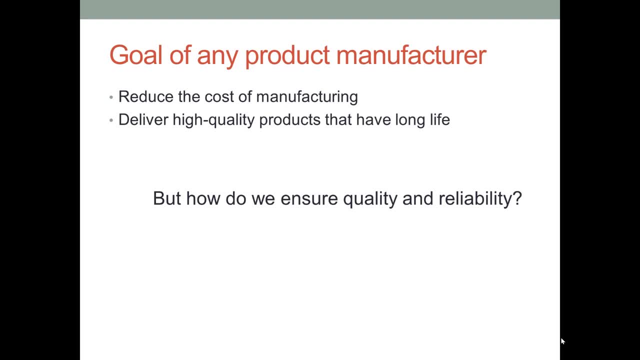 we say that the defect quality or the product quality is 100 defective parts per million or DPM right. So usually you would like to minimize that number. So 100 is a number that has been around for a while, but with markets such as automotive or industrial systems, that number 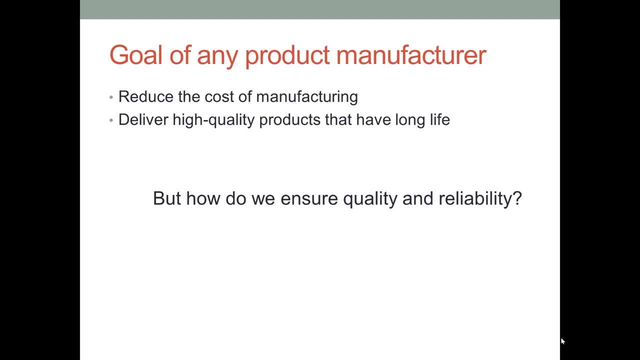 has come down very drastically. So today we talk about DPMs, which are less than one right for products which are expected to be used in situations like automotive or industrial systems, where you know there may be robots or, let us say, 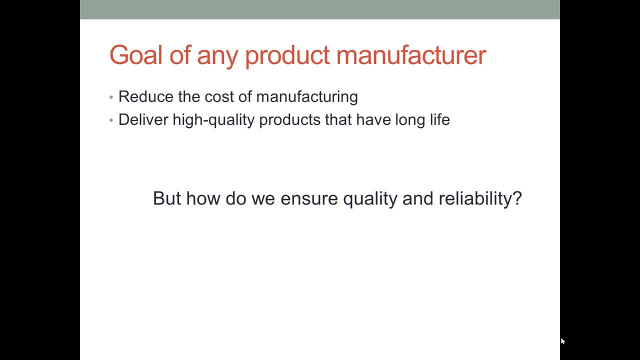 somebody is using some electronics in a car, So the life of a person may be in danger If product does not work correctly, right. so that is the reason why people demand extremely low defective parts per annum. not only should the part work at the time when it is sold. 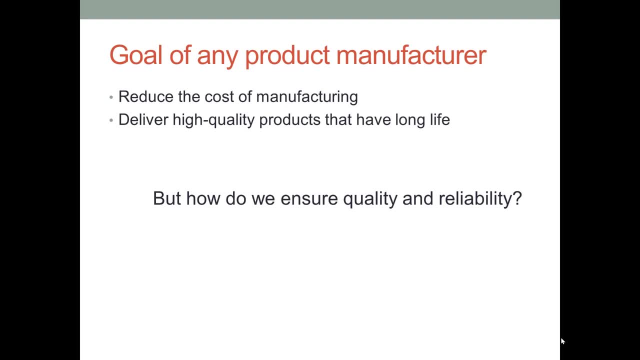 it is also expected to work until its lifetime, right? so there is always a warranty that comes with any product. so suppose we have sold a product for five year warranty period and the product fails within that warranty period, then i know it is, you know, bad for the supplier. 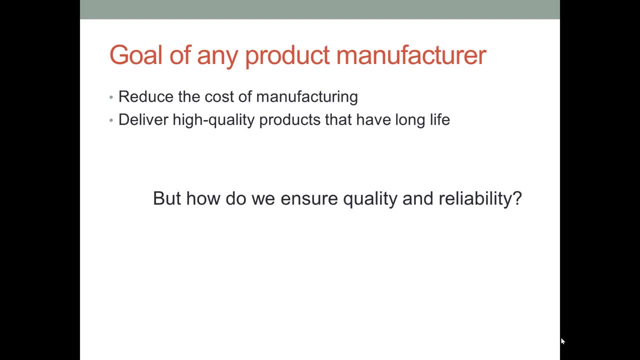 because you know it is a problematic situation. right so we want our products to be not only of high quality, but also of high reliability. right so that is our goal. so from the- you know- design designer side, from the manufacturer side, all the way to the consumer- right, there is a big chain of events that takes place, right? 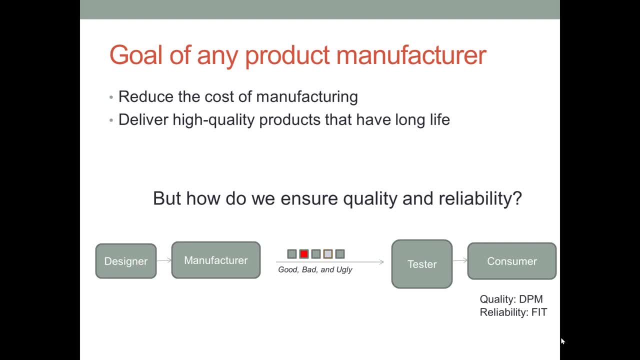 so sometimes the design and manufacturing is at the same site. but in a distributed situation it is quite possible that the design activity happens in one company or in a different site of the same company and the manufacturing happens somewhere else. so the first step is usually the design step, and then you know, the product is manufactured and we make a large number. 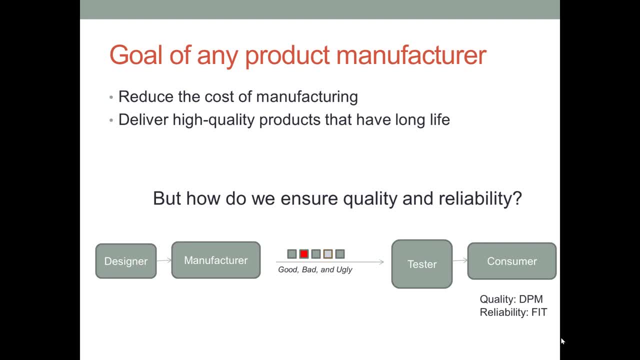 of these products, and sometimes some of them are, you know, bad products, meaning which are going to fail right possibly at the manufactured. supply rates and manufacturing rates sometimes side itself right if we are lucky, if that happens right, I mean if the manufacturer discovers that there is a defective in the part, defective in the 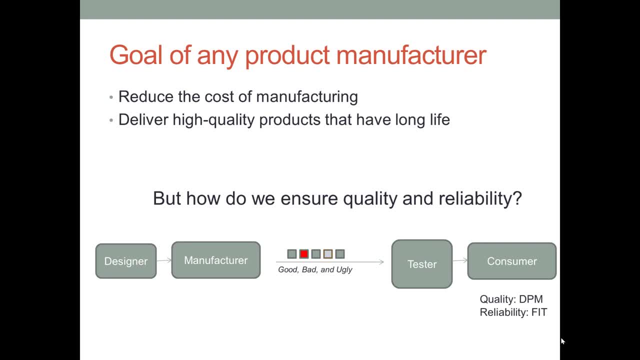 part, then he throws it out and he doesn't sell it to the customer. but it can be an ugly situation where we did not discover that defect at our end, at the manufacturer's end, when we sold it to the customer, and then you know the customer discovered it, used it in the part, and that can be a sort of a sad 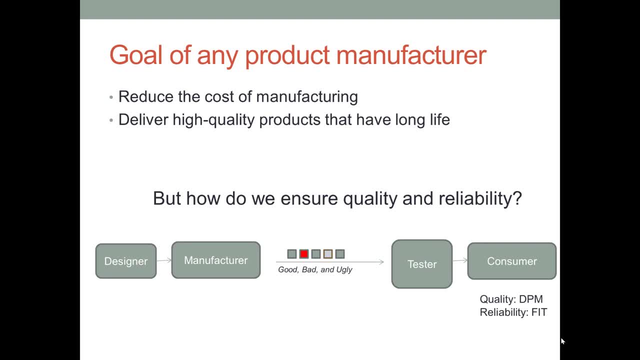 situation right. so I already mentioned you about the DPM measure. in the same way, there is a measure for measuring the reliability, which is sometimes called the fit measure or the failure in time. so usually we look at a certain number of hours, a very large number of hours, and say: you know, we do not want. 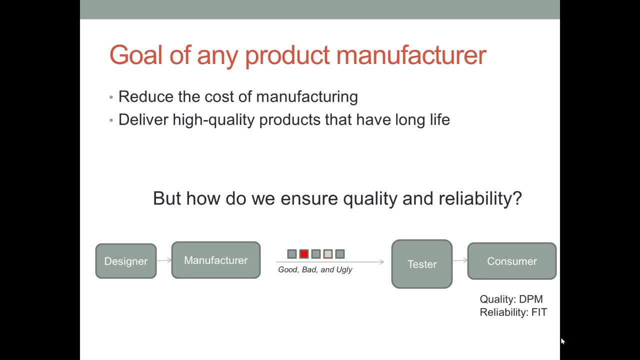 that A even one fault to occur in so many hours of operation. so that is how usually fit is measured right. so now that we have understood what is quality and what is reliability, let's try to understand the impact of, you know, failure. so if a customer finds that the product does not work right, then the 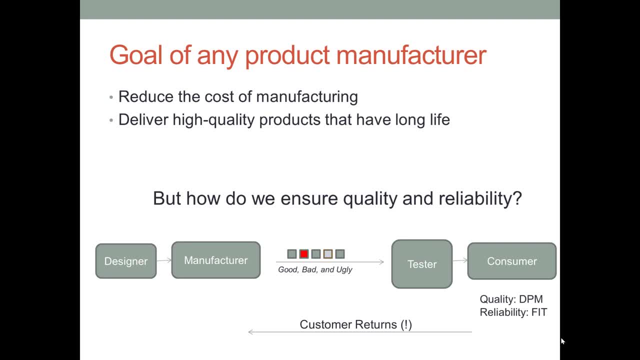 customer has every right to return the part, and that is a nightmare for any product manufacturer, right? so we won't like to see that happen, because it requires a great deal of- you know what we call, as you know, debugging. we have to find out what exactly went wrong, if there is a defect at all, or was it? 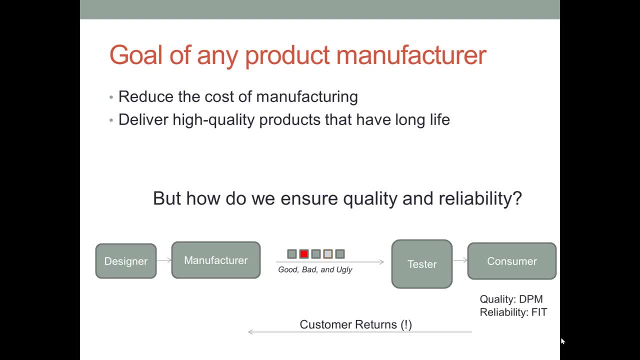 because the customer did not use the product the way it was supposed to be used? and if there is indeed a defect, what caused it, so that you know we call that as failure analysis, so that we call that failure analysis. failure analysis is a very time consuming task, So we don't really, you know, would like we would. 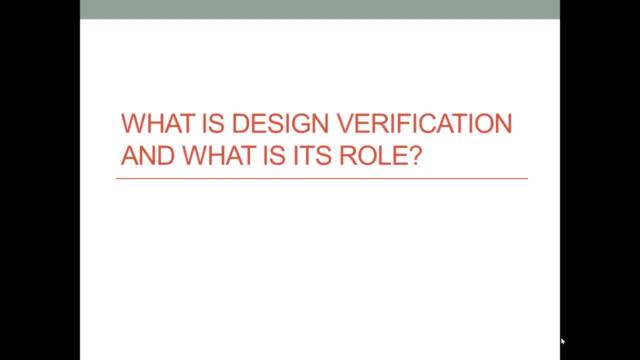 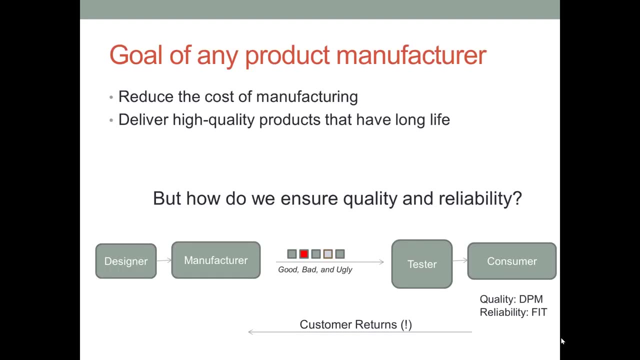 try and avoid getting into those kind of situations, right? So let us first understand what is design verification and what is its role in all of what I just told you, right? What role does it play? Obviously, our goal is to improve the quality and reliability, and that is where, hopefully, design 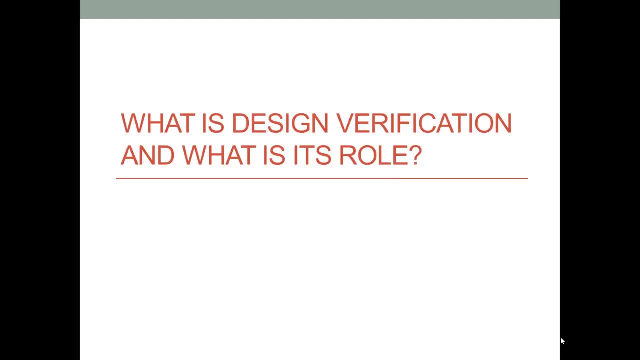 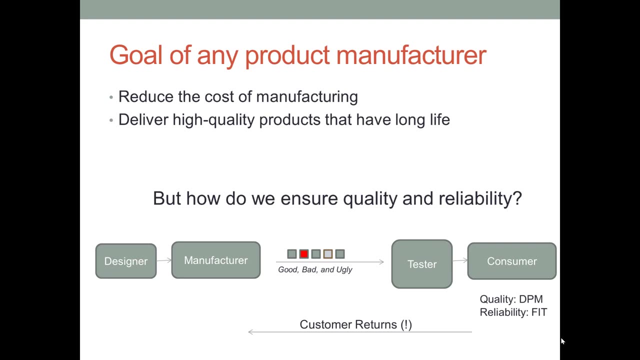 verification will have a role to play right And, by the way you know, it doesn't mean that verification is the only way we can get reliability and quality. There are a lot of other steps and all of them need to be sort of. you know, they are all collectively responsible for maintaining 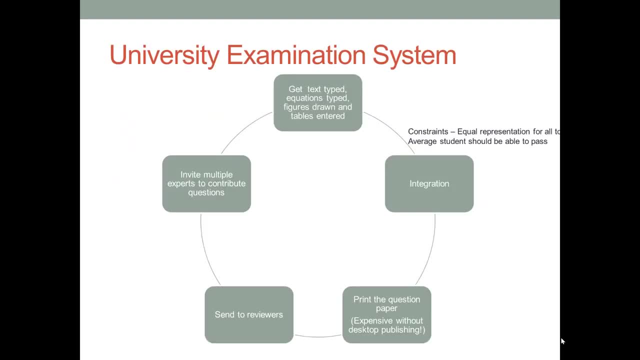 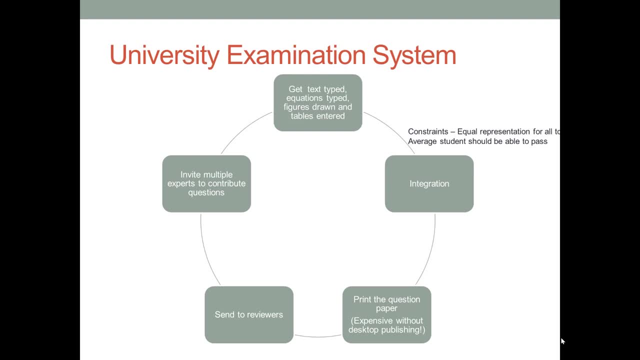 location: espresso. So if you are a bathroom student, I'm sure you have taken examinations, and if you belong to a large University system with many colleges, the sort of task of conducting such an examination is quite laborious because there are so many colleges. 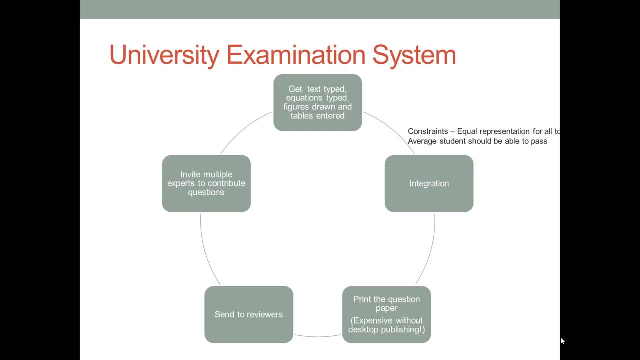 maybe hundreds of colleges and in each college they may be hundreds of students. So a large number of you know question papers are required to be printed. you know, and imagine that you know there is an examination and in that examination you know when we distribute. 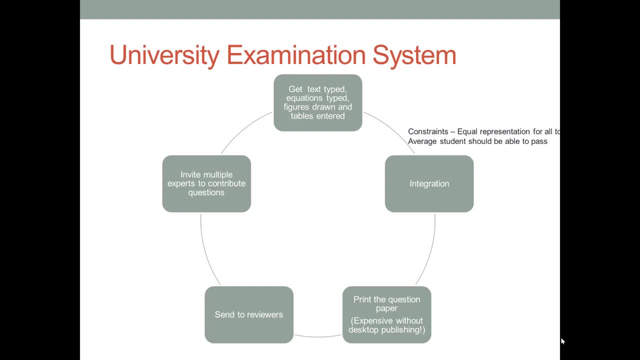 the question papers. somewhere in some college there is a defect in the way that question paper was printed. maybe right, maybe there is a blank page or something like that. there were supposed to be two pages and one of them never printed, or maybe you know, something didn't print well. 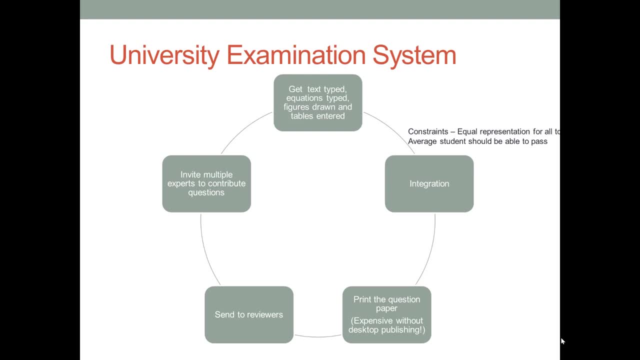 right. so these kind of defects could exist and if the student realizes it right and points it out, maybe there is something that can be done. you know the an alternate question paper copy can be provided to the student. but what if the student never realizes right, if there is an empty? 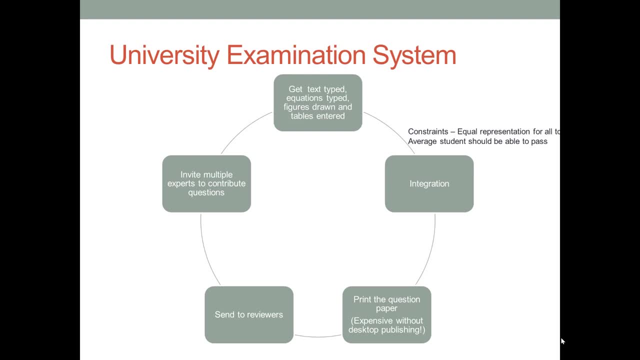 page. I don't think the student may realize that. you know there is a bunch of questions missing, so that can be a very problematic situation, right? similarly, what if there is a problem in the way the question is framed? right? I mean, there is a possibility that it was not interpreted properly, right? I mean there are two or three interpretations of the. 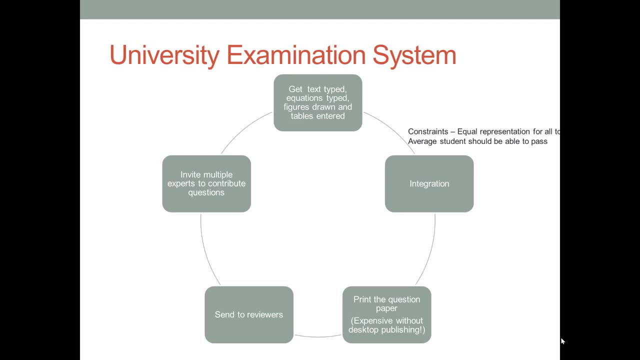 same question and everybody you know makes a different assumption and they all come up with different answers, and that is going to be a nightmare, right? so for anybody who is correcting the- you know, the answer scripts, it can be a major problem, right? so, as you can see, there are two types of problems here. one is where the question paper had a bug, so 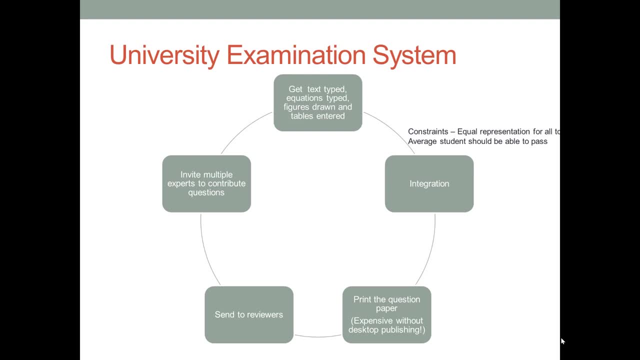 to say: what is a bug. it was a situation where the person who wrote the question did not, you know, spend enough thought in writing down the question in an unambiguous way, so maybe certain things were not specified properly, so that means there are multiple interpretations possible, or? 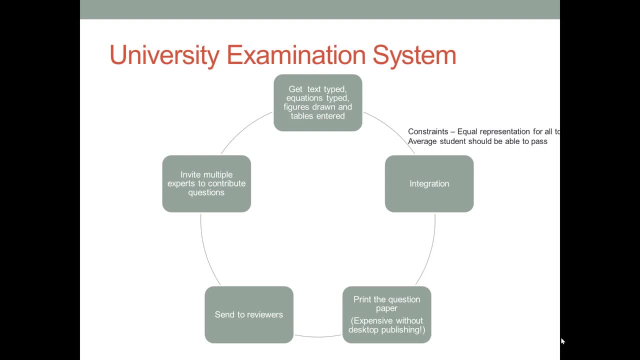 there is just a error in the question. right, the value is incorrect. you know, maybe some value is missing, some value is incorrect, right, so we call such a thing as a fundamental bug, right, or a sort of an error. right, so this can happen in a design as well, right, and an example. 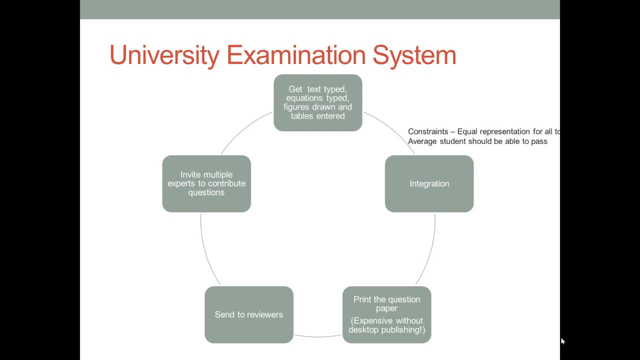 could be. you know, you have a design in which you know there is a possibility of a incorrect answer being generated, right? so you know, imagine that you have designed a chip for some arithmetic right, and some times it gives the incorrect answers right because of some bug that is present in that. 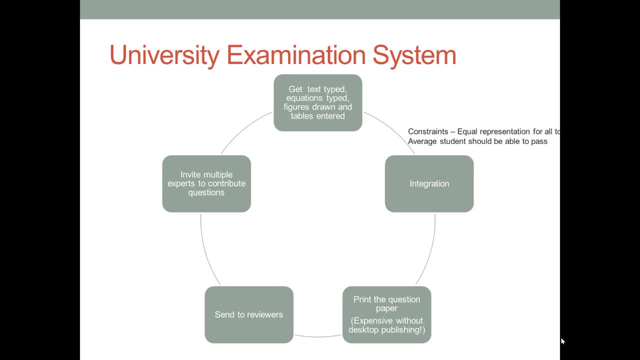 algorithm that has been used. it produces an incorrect answer. right, so that is a functional bug, right? so how do we eliminate this bug? obviously, we have to do a lot of design verification. so design verification is basically a way to remove functional bugs. so, in the examination system, coming back to the analogy that we were discussing, what do we need to? 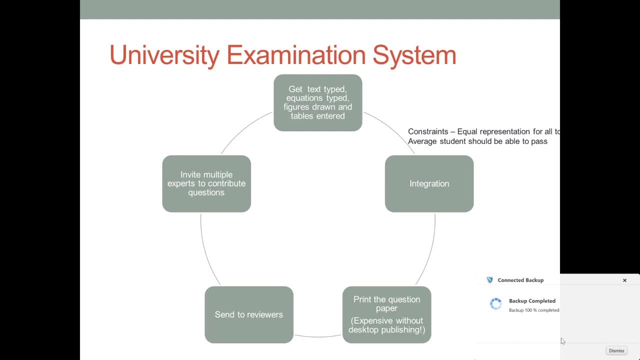 do we need to have a committee, perhaps right, which looks at all the questions, right, and they, you know, simulate that environment. they put themselves in the situation of the student who is reading those questions and look for any wrong interpretations that could occur. is there enough clarity in the question? is some value missing? are there grammar errors? are there? 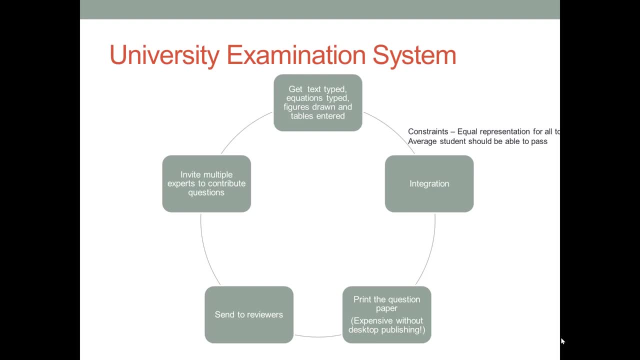 any typographical errors. is some chart supposed to be provided with the question and it is not provided. some data is missing. so people go and do that quote-unquote simulation, right. the same thing has to happen in the design context, also through some sort of a simulation. 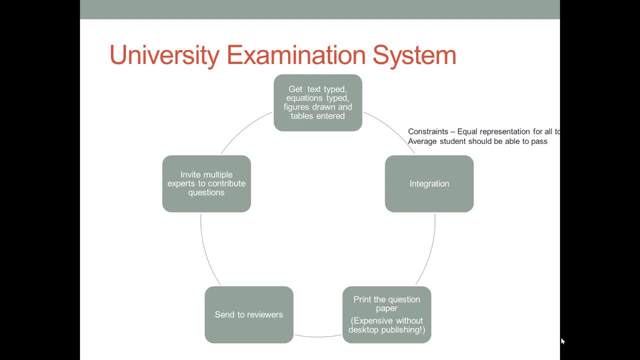 we need to figure out if there exists a bug in the functionality. all right, so how do these bugs enter right the inter? because many people may be involved in creating the question paper. so sometimes what happens is, you know, people form a community. right, there are a bunch of experts. 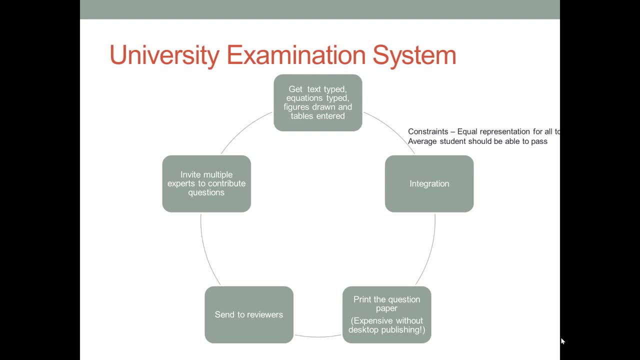 who get together to suggest questions, right, and sometimes they may just write the question on a piece of paper, right, and somebody else comes along and types those questions into the question paper, right, and this is a lot like the way designs are done today. design houses are geographically. 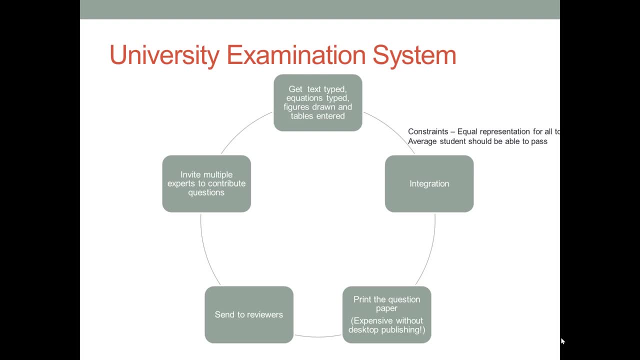 distributed and a lot of reuse happens, right? i mean, you know, today there is no time available to sort of design everything from scratch, so a lot of design reuse happens. so when you reuse what is already present, right, and you don't pay attention to the proper integration, then there is a chance that there can be a bug, right, so design bugs can enter. 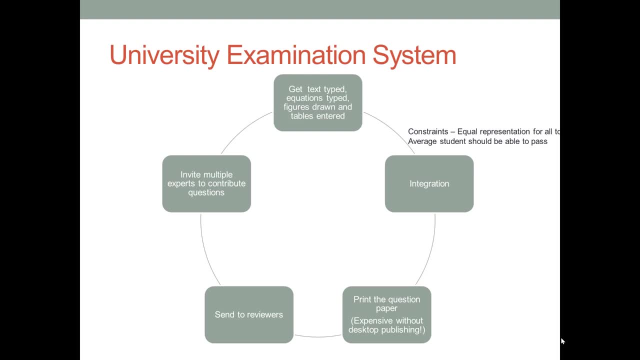 in so many ways, right. so in the examination- sort of analogy, what, if you know? the professors suggested a number of questions and when they finally made up the question paper, a particular chapter was never accounted for, right, and there were too many questions from the same chapter. that is an example of a functional bug as well, right so, or you know, 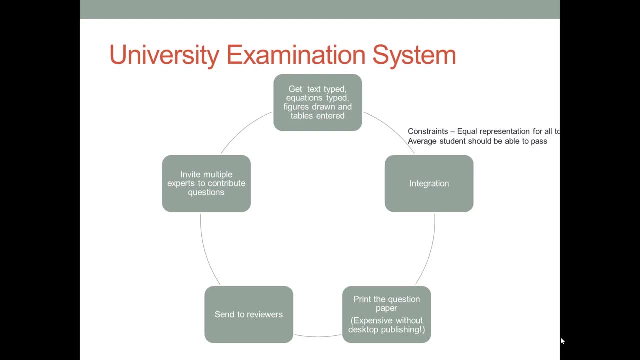 when the equations were typed, there were mistakes, things like that, right? so, like i said, the only way is a thorough review, right, more than one review may be required, and then maybe these functional bugs can hopefully be solved, all eliminated. But, as you may have experienced, one can never eliminate these bugs all together. 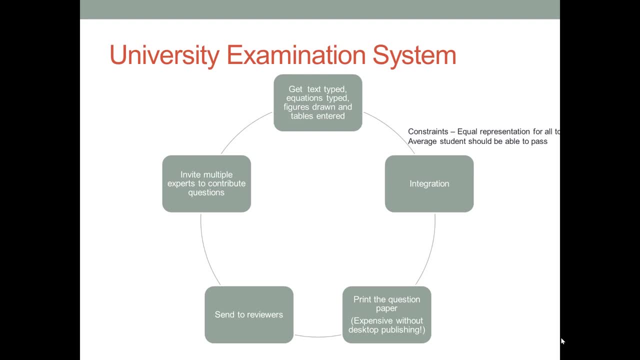 There is always in any examination system. occasionally there will be some sort of a bug like this which causes a lot of problems for students. And once the verification is over, once we are happy that the question paper is good. it has a fair representation. 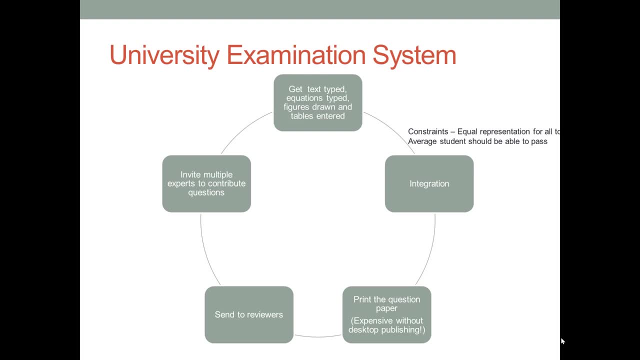 for all the chapters. there are no bugs in the sort of way the equations were typeset and everything is all right. So usually at that stage we are willing to give a print, And today, luckily, we have what is called a desktop paper. 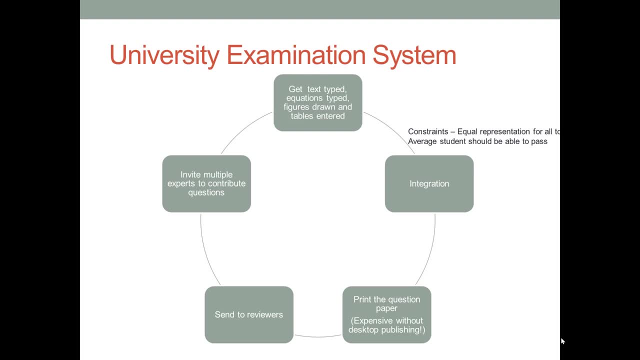 We can just go and print a couple of copies of the question paper. That was not the case a long time ago. We used to depend on a printer, So we had to actually send out the question paper in a handwritten format to a printer who would actually do all the typesetting. 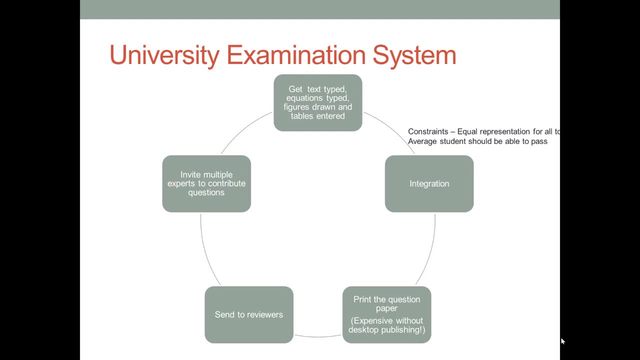 and then he would return what we call as the proofs. So let us say: the proofs come, And then you would realize that there are bugs there. Something is not printing properly. You have used a Greek character, gamma, and it does not print the way you expect it to. 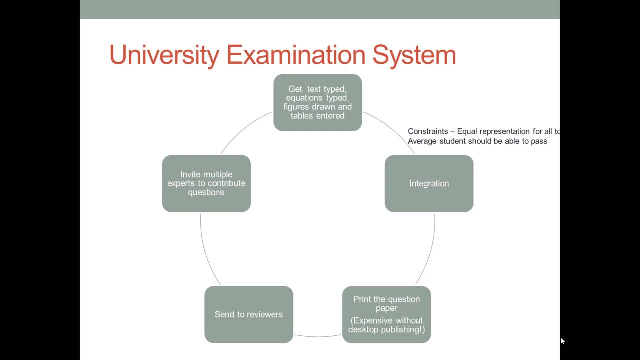 print, Or some suffixes are wrong Or the superscripting is not printing properly, or something like that. Notice that this can only be done post printing Up to this, And then you know the activity of designing the question paper, sort of reading those. 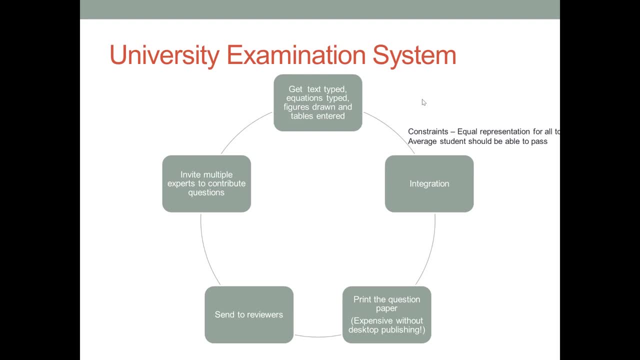 questions. you know, on the screen. Right, We are not really printing anything yet, We are just reading everything on the screen. Maybe we are mailing the questions to one another and things like that, But everything is still on the screen. Nothing has been printed. 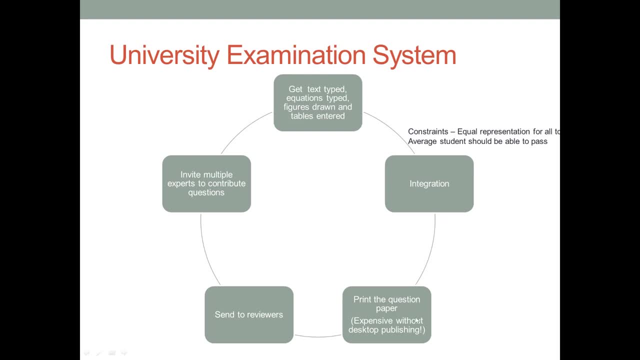 yet Right, And here we have actually taken a copy of the question paper And we have actually done a couple of printouts and we are looking at. you know what the printed question paper looks like And when we are satisfied, you know we go and tell the printer: it is okay to now print. 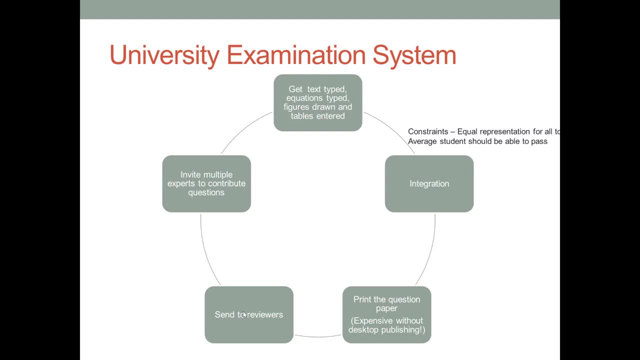 in large numbers. Maybe we want 100,000 copies or 10,000 copies of these question papers. So, as you can see, there are three distinct stages here. Right, The first part which I mentioned is what we call as the proofs. 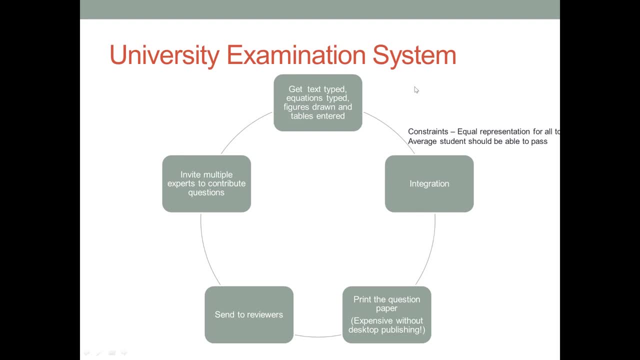 The verification Right, Where everything happens before, even you know, going to the printer. And then there is a part where you know we have just printed a sample question paper, Just a few samples maybe, And then we are looking at it, Maybe we distribute it to the 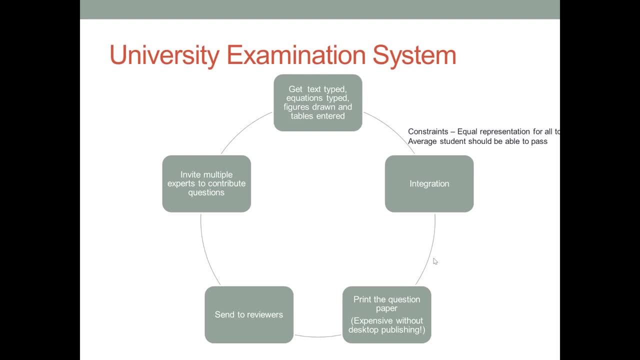 entire committee And then they all look for you know there are any printing mistakes and things like that And they are fixing them Right. And when they say it's okay, you know we go and you know produce it in bulk, Right. 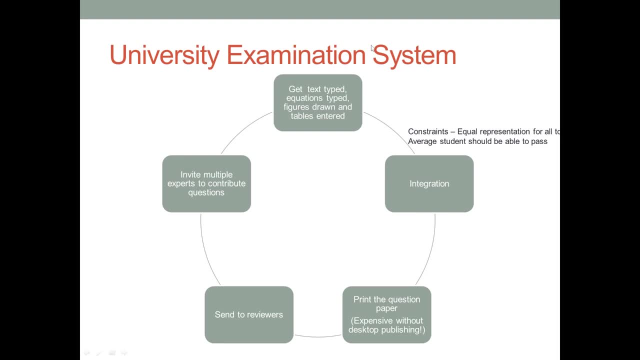 So this part is sometimes called verification Right, And then this part is sometimes called validation Right, And then when we get it in large numbers- maybe you know we have got a whole bundle of maybe 10,000 questions, question papers- then can we trust that everything? 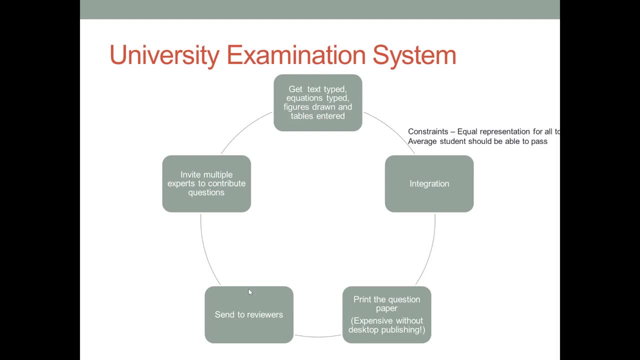 has gone well there. Right speaking, that may not be correct. also, right, I mean, I have a every possibility that when we make such a large number of question papers printed, one or two somewhere may have a problem, some defect. right, it happened because you know, when the printer was printing maybe some paper got. 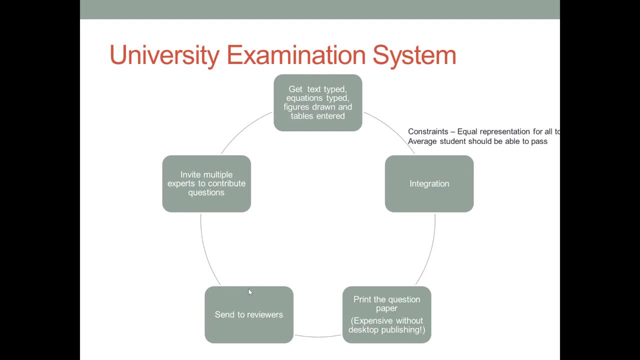 jammed and it was cleared. or maybe, you know, the inking was not perfect. whatever. maybe the reason that was what is called as a manufacturing defect. it has nothing to do with the functional bug. right, we had verified all the functional bugs and we thought everything was good, but unfortunately, 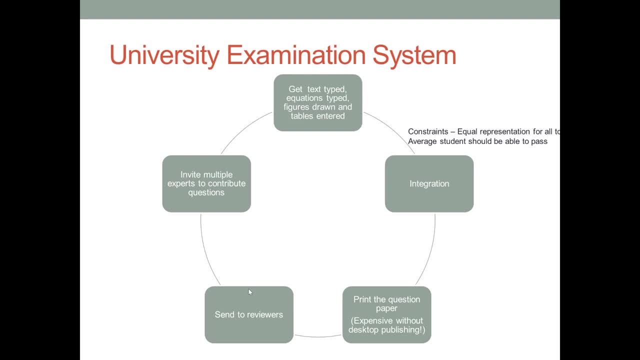 some manufacturing defect entered, not in every one of them, but in some of them. so the nightmare of the functional bug is that if it is there, it can get duplicated in every, every part, right. so if I am a semiconductor manufacturer and I make millions of these ICs, 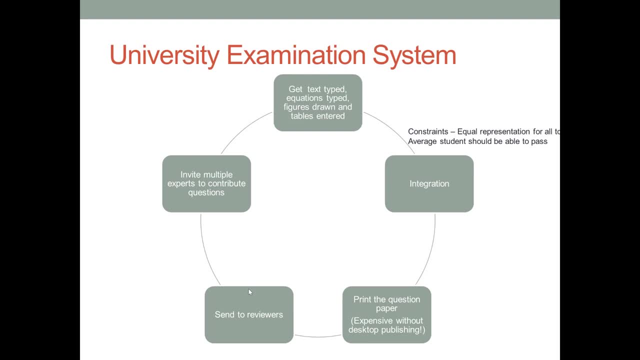 and if there is a functional bug, unfortunately it should be duplicated in every one of those million parts, right? whereas if I have verified it, well, right, and then I am doing a manufacturing. the defects do not enter in all of them, they are randomly in here a little. 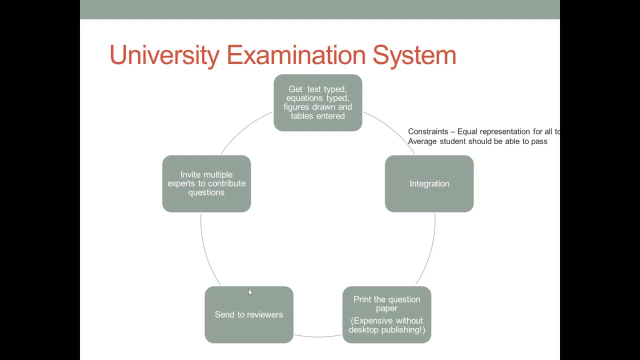 seja to be 還 in the parts which are bad and only sell the good ones to the customer right. So that is called testing right or manufacturing testing right, and that is a you know very labor intensive, very, you know high cost. you know activity right. 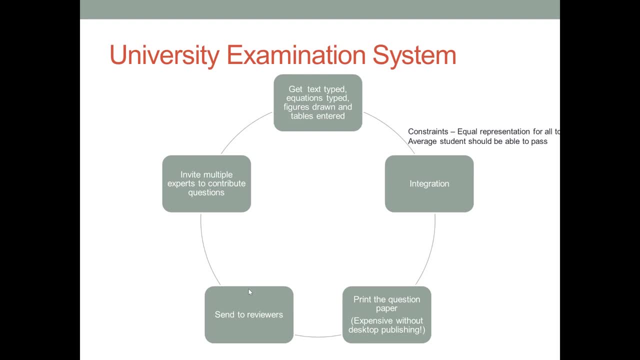 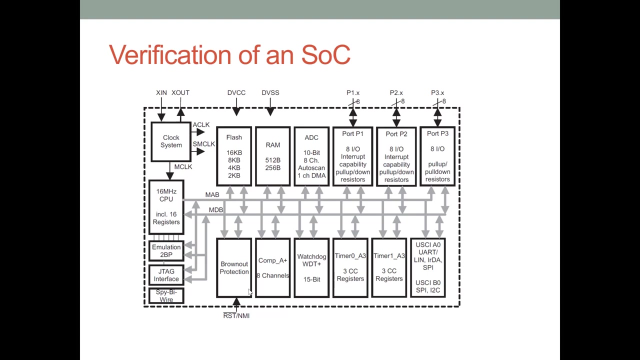 So you can imagine that all of these three things that I mentioned, they have an analogy with the analogy of the examination question paper system. I have tried to explain. you know what these three steps are: verification, validation. So today, let's come to you know, let's come to today's systems on a chip. 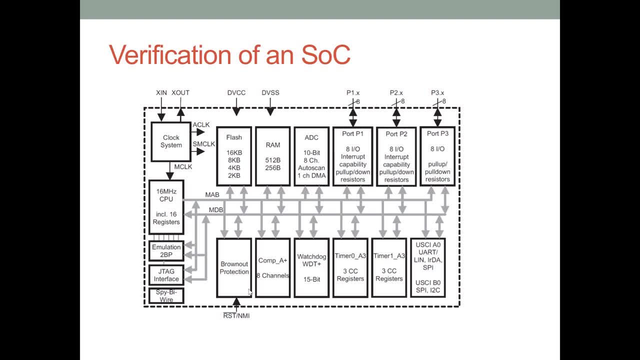 They are very complex right, and I have chosen a very simple example Here: the TI MSP430. it is one of the very simple embedded processors which has got a 16 bit CPU right and it has got some built in embedded memories right, and it has got 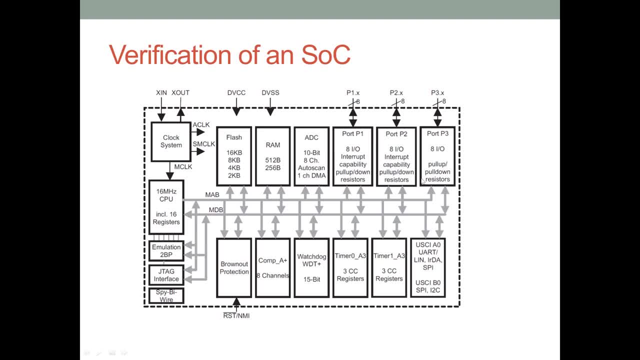 some analog to digital converters, some IOPORTS. it has got some things like timers, watchdog timers, and then there is some communication peripheral right, and then there may be some, there may be power, you know, management, kind of a peripheral brownout protection. there may be some comparators, analog comparators, all these kind of you know, we call them as. 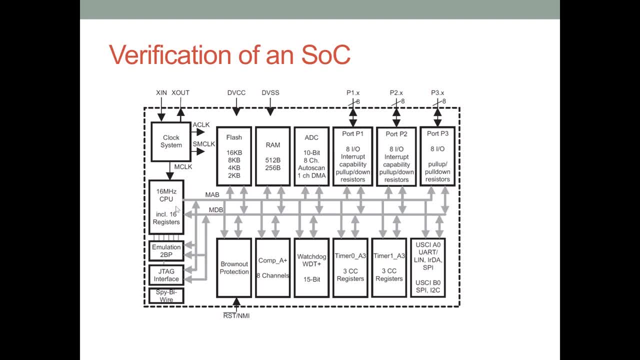 IP right. There are a number of these. you know some of them. some people use the word subsystems for these right, or IP, whatever you call them- intellectual property right. So in an SOC today, A modern SOC Right, A modern SOC will have easily hundreds of these IPs right. 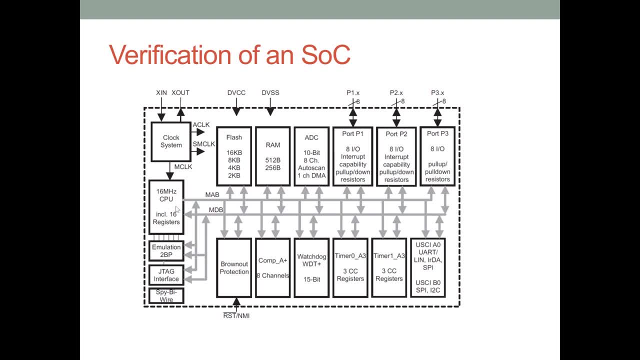 That is why the design complexity is very high and you know the person who is selling this SOC after manufacturing, that SOC sort of takes responsibility for supplying you know a part which has no functional bugs, which has no manufactured defects, which has no you know defects post manufacture. right. 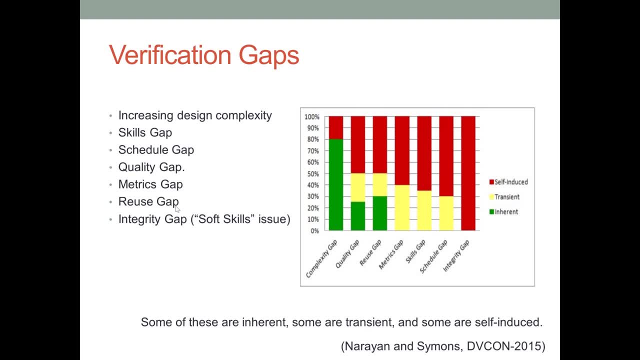 So there are, unfortunately, in the process of verification there can be many problems, and here is a you know paper that was published in DVCON 2015. DVCON stands for Design Verification Conference, So in a recent paper published there, the authors sort of make a nice case for various gaps. 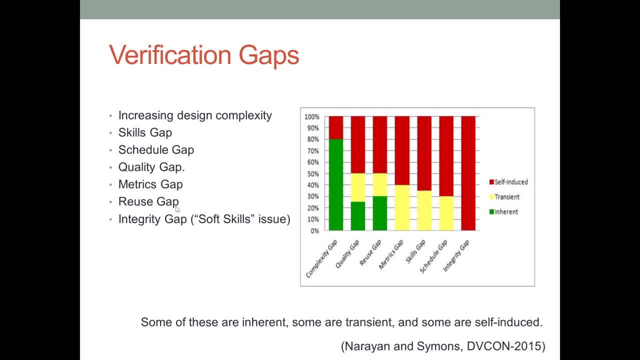 that can exist in the process of verification. One, of course, is the complexity of the design right, So you may be surprised to know that you know to verify such large SOC, the number of people involved will be very large right. So a lot of people get involved in design verification right. 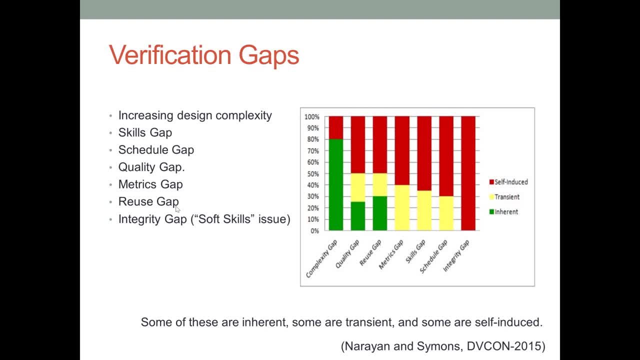 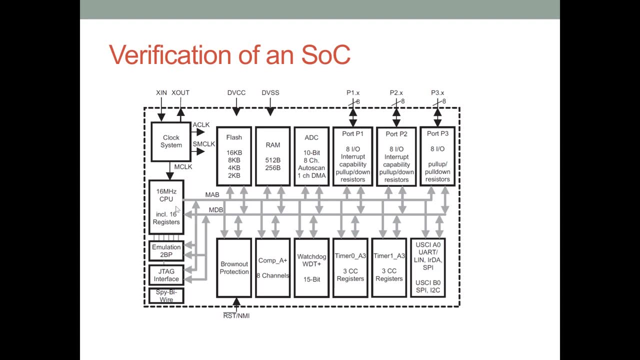 And they may have skill gaps, see, because not everybody understands all the IP right. So, going back here Sometimes, Sometimes you know you are not a domain expert in the area of signal processing but you may have to verify a signal processing IP right. You may not be a domain expert in image processing but you know you are being asked to verify. 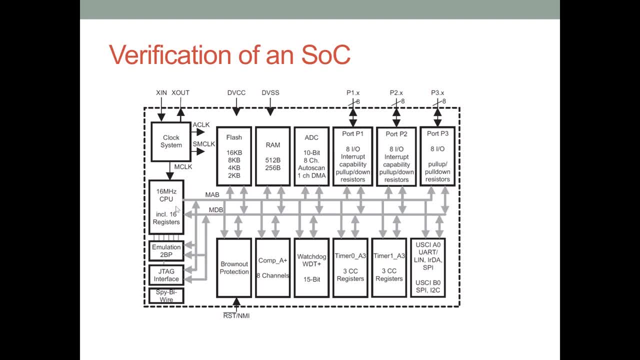 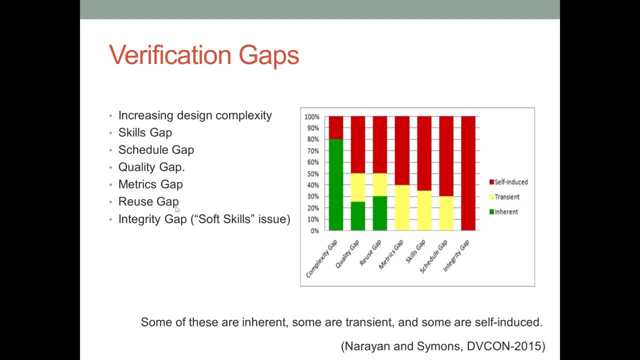 an IP that does image processing right, And there are so many different areas right- communications and signal processing. there may be some computational blocks, So there are so many different domains to which an IP may belong right, So there may be a skill gap. there may be a skill gap in terms of the usage of tools, right. 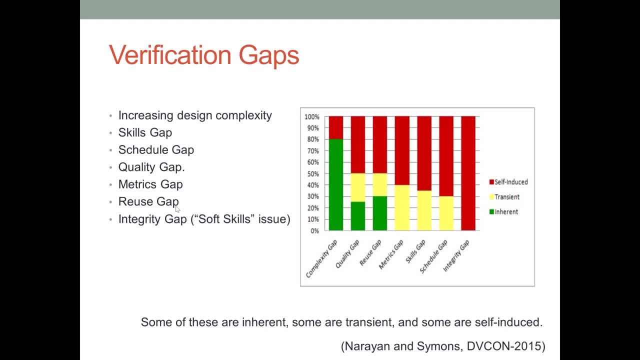 Then sometimes there are scheduling pressures, right, People have to plan out the entire verification how it is going to be done, etc. So there could be a gap there Sometimes. You know there are, You know There are some unwritten rules about quality. 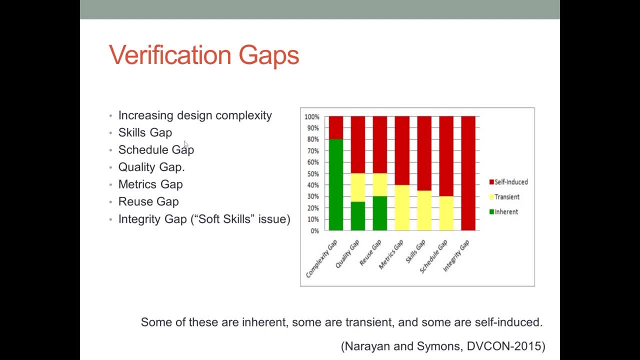 People didn't quite understand what was the coverage required and things like that. So there may be a gap there in terms of quality, or rather the understanding of you know quality. similarly, metrics right. When I say metric, it could be you know how much verification should we do, right? 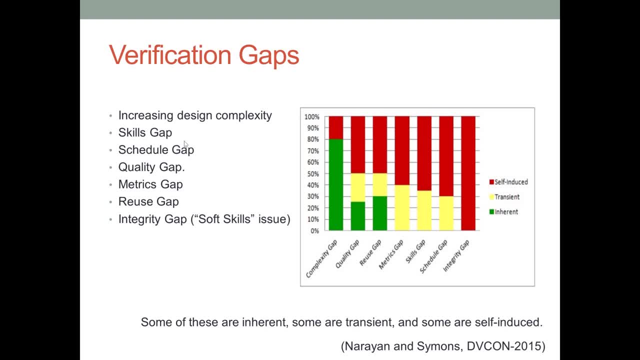 If you think about it, if you take a digital system, verifying it exhaustively is impossible. The complexity of the IC or the SOC is so large that there is no way we can verify it exhaustively. So we had to pick and choose our test cases, right? 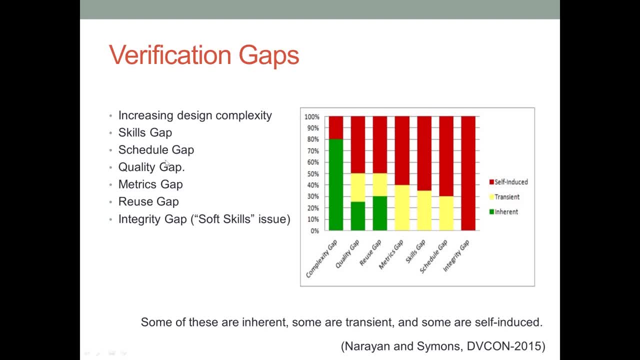 So when we do that, there is a possibility that some of the bugs may never get discovered. So people are worried about how much verification are we doing? Are we doing enough right? So there is a concept of coverage that people try to use to define. you know the quality. 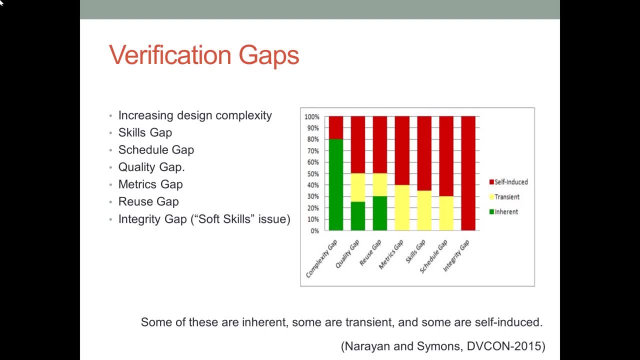 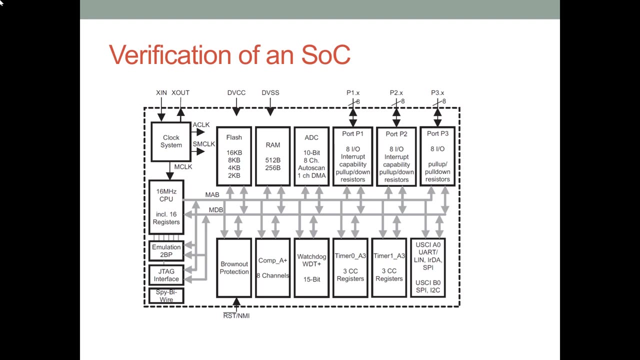 of the verification. So not understanding what these metrics mean can result in a gap. Then the reuse that I talked about. see, there was a time when everything was designed from scratch, right, So the whole IC was designed as a custom IC. People used to design everything from scratch. 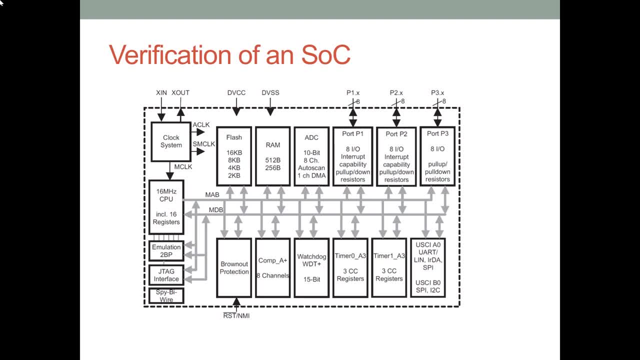 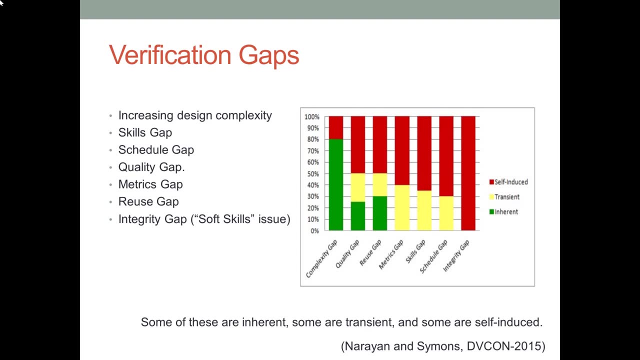 So then you know, people can be more careful, maybe in terms of the interfaces and things like that. But when you cannot do that, when you are relying on reuse of IP which you may have purchased from other companies, and so on, there is always some little bit of- you know, gap there in terms. 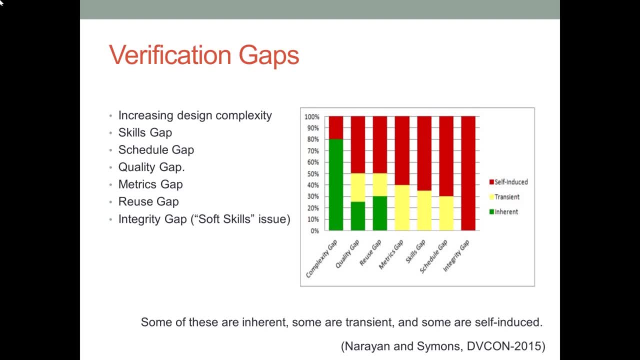 of the IP reuse and not having enough documentation and things like that. And finally, There is also a soft skills issue. I mean, sometimes people you know develop an attitude- and this is what the authors point out- that many times either it's a designer or the verification engineer: verification. 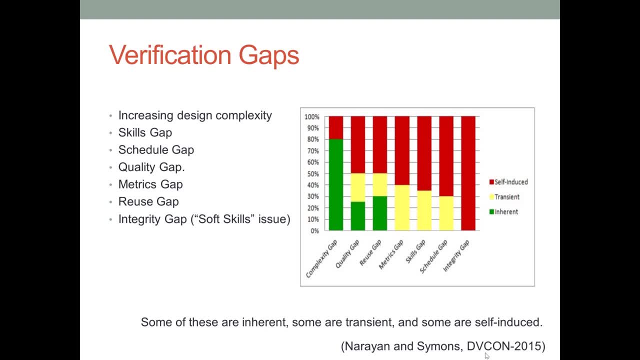 managers, design managers, they may all sort of have a quote unquote integrity gap which results in some amount of loss. So You can see that this is what they report. So the red part is the self-induced part. that means this gap was induced by my own attitude. 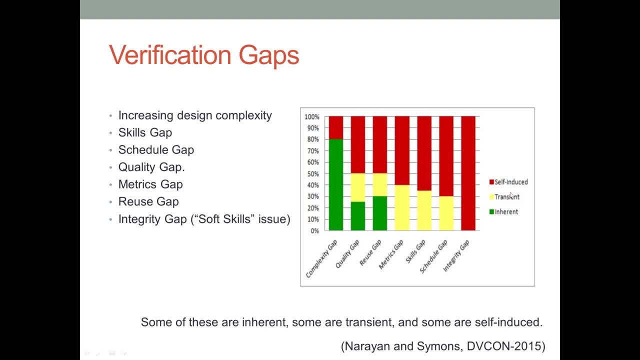 by my own thinking. Then there is an inherent gap. inherent gap means you know it cannot be eliminated at all. You know nothing can be done about it. Take the design complexity gap. a large part of it is true, It is. It's a. 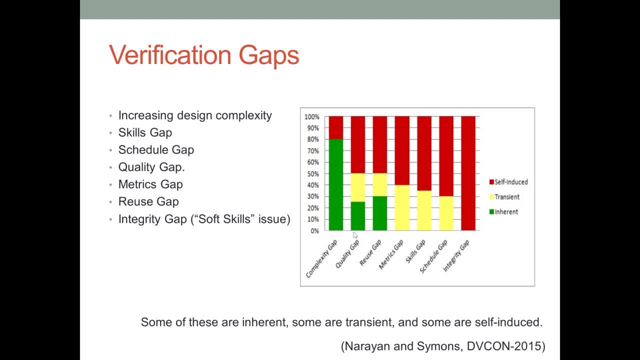 It's a problem. We are designing more complex sizes than ever before, So it's an inherent complexity, but there is a little bit of, you know, a self-induced gap there as well, Right. On the other hand, take the integrity gap. it is entirely, you know, made by us. 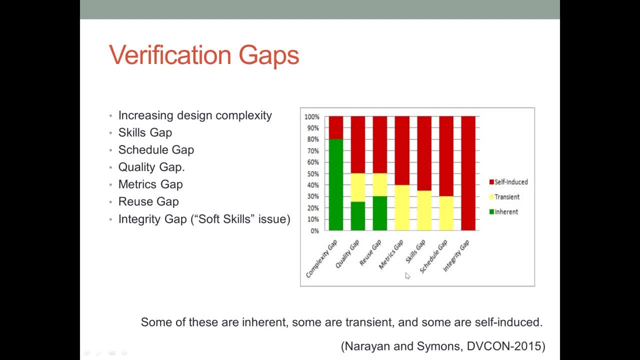 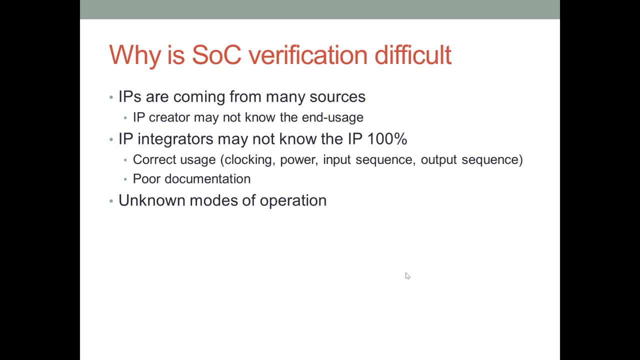 It's a self-induced gap. So interesting paper. You may want to take a look at it. So, going back to why is verification such a challenge? I hope everybody understood The role verification plays. it is to eliminate all the functional bugs. So we are not talking about timing at this point. we are mainly talking about functionality. 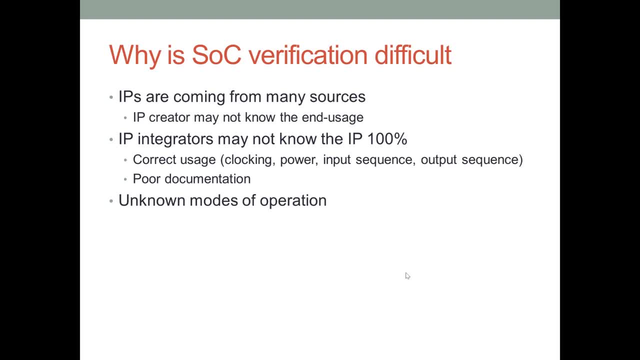 We are worried about. you know bugs such as you know. maybe, like I said, you know an arithmetic that may not happen. correctly. Right Results are incorrect. Right, I'm sure you have done this in your examination also. Right. In an examination there may be some complex calculation that you need to do, and because 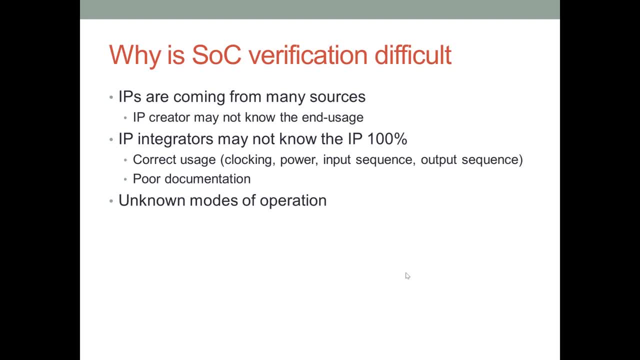 of you know some speed at which you are working. you may have made some error, So you go back and do it again and you are getting a different answer Right. So you go and verify what went wrong and things like that. So that is what verification is: to verify whether the intent has been correctly captured. 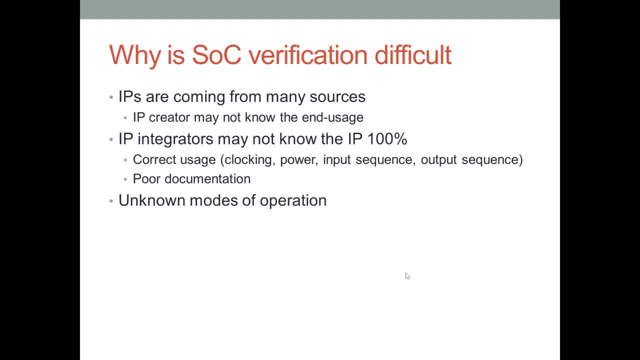 So we refer to what is called as a spec Right? So somebody wrote a spec for us saying: you know, this is what the design must do, and then the design engineer took that specification and came up with an implementation, and we have to verify that these are indeed the same. 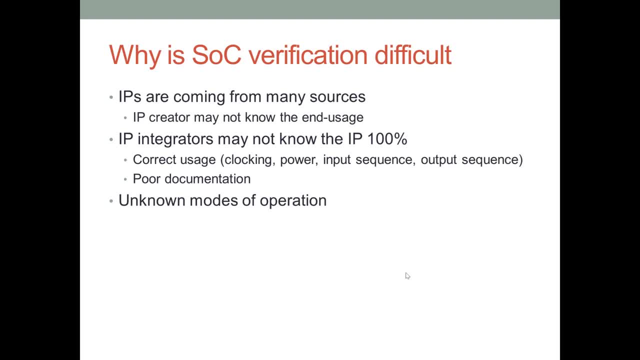 So the verification engineers role is to verify whether the design is doing what it is expected to do Right. So the challenges that the verification engineers may face are: see: the IPs are coming from a number of different sources, as I mentioned earlier, there may be different companies which 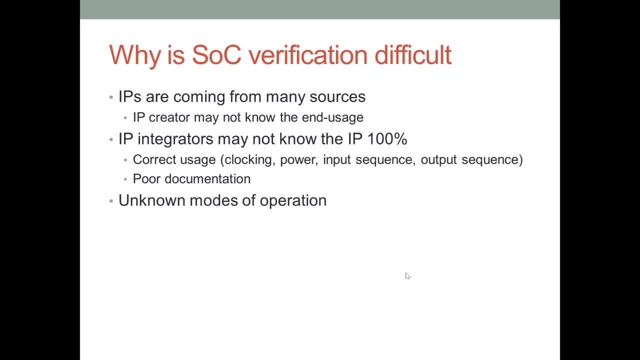 are providing these IPs, multiple teams involved, not maybe enough documentation available, and the IP user and the IP creator may not understand the end usage Right. The person who created the IP may have made assumptions and actually may have forgotten to document those assumptions on paper. 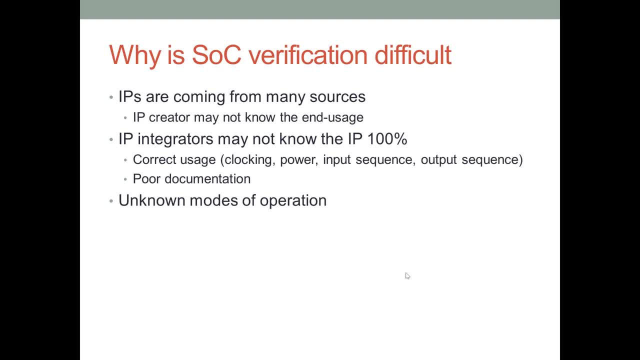 Right. And the people who use that IP. they think that it does things in a certain way, but it doesn't Right. Then, similarly, the IP integrator, one who integrates all these IPs into SOC, that person may not fully understand the IP Right. 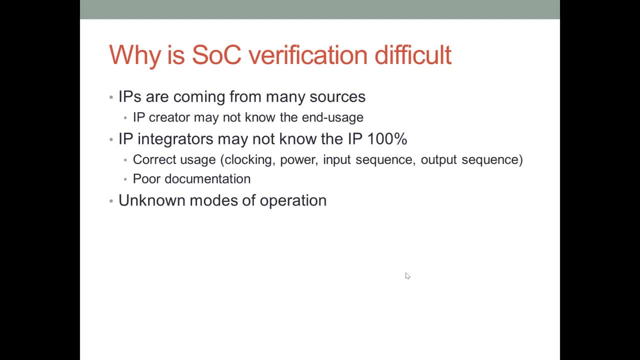 So he may not understand what is the correct locking mechanism to be used, how much power it consumes, or you know what is the sequence in which it must be powered on. You know what is the way an input must be provided, in what sequencing. similarly, how is the output? 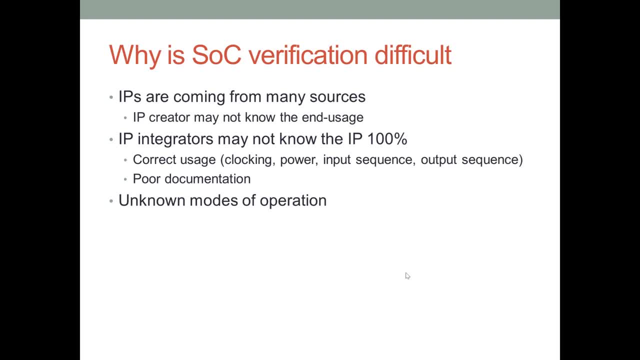 provided by the IP, etc. Right. And then there may be modes of operation which are unknown as well, Right. These are not written down anywhere and all these may result in the verification engineer may not be in a position to verify the IP to the best of his or her knowledge. 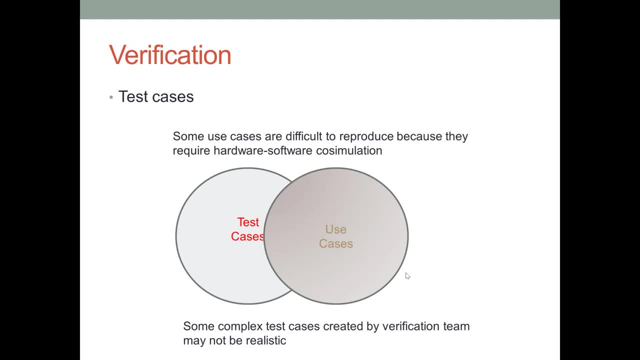 So I mentioned the word test case earlier also, Right, Sometimes it is called the test bench, So people who are in verification, they are asked to write these test cases, Right? So imagine that you know. there is an example of a addition, Right. 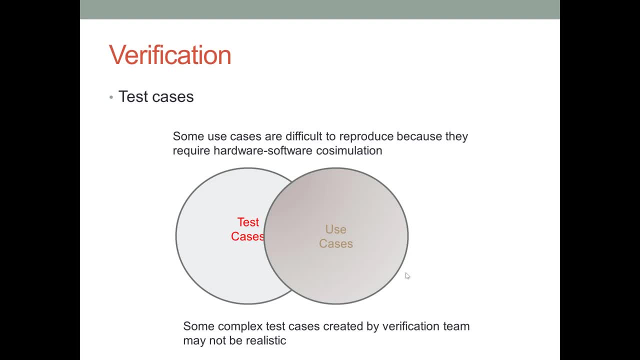 There is a very simple example of a 32 bit adder or something like that: Right, So if two 32 bit numbers are added, Right, So each of them can take 2 to the power 32 combinations. Right, I mean each input can be any one of the 2 to the power 32 numbers. 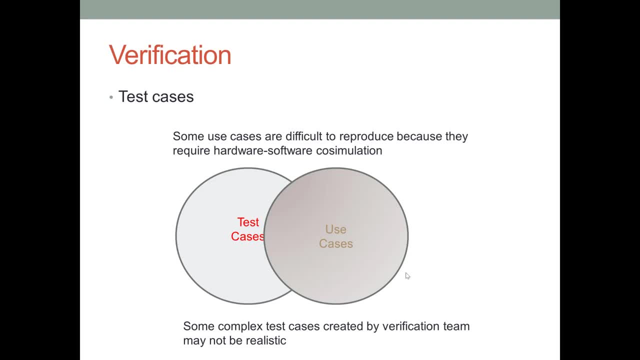 And obviously you cannot, you know, go and create that many test cases, Right? It is not required as well. Right, You have to look at what is a representative case, Right? So that is what verification engineers are actually going to do, Right? 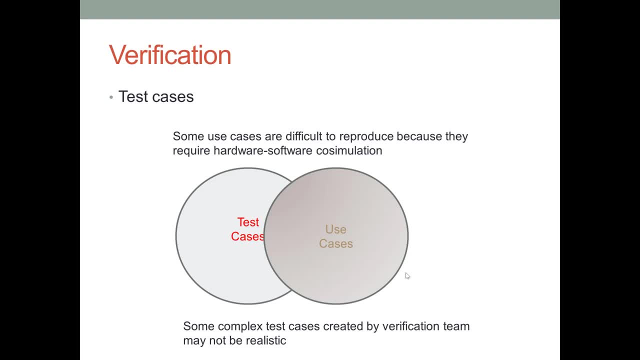 So they created a whole bunch of test cases. Obviously, the more test cases you create, the more confidence you build, Right? But that also would mean a lot of run time. See, remember, verification is mostly a simulation activity, Right? So we do not have any chip in place yet. 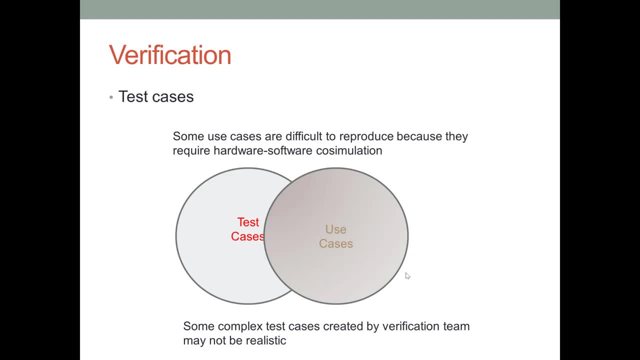 We do not have any chip. We just have maybe the Verilog Or the VHDL model with us And we are just simulating that Verilog or the VHDL model, Assuming that everything else will work Right. We assume that when it is manufactured it will be all right. 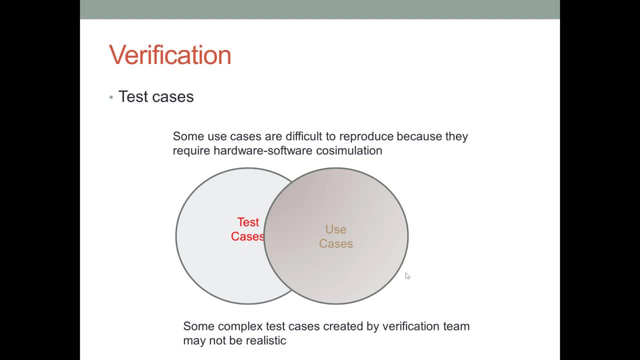 Right. So that is what functional simulation is all about, Right? And what about the usage, Right? See, I have shown here 2 circles. One represents the set of all the tests that we have written And the other represents the set of all the actual tests. 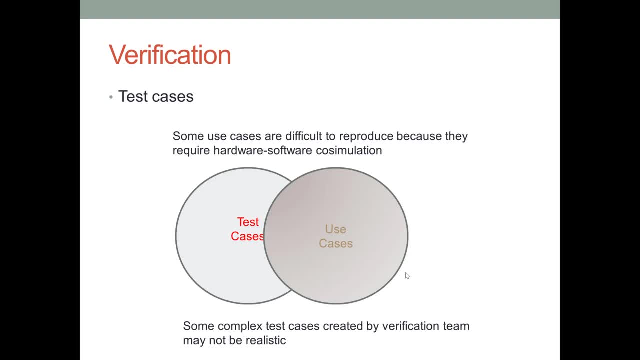 Right. So the intersection between these 2 circles, You know it should be as large as possible. Right, Because that means there is a use case and there is a corresponding test that has verified that the chip will function well under that particular use situation. 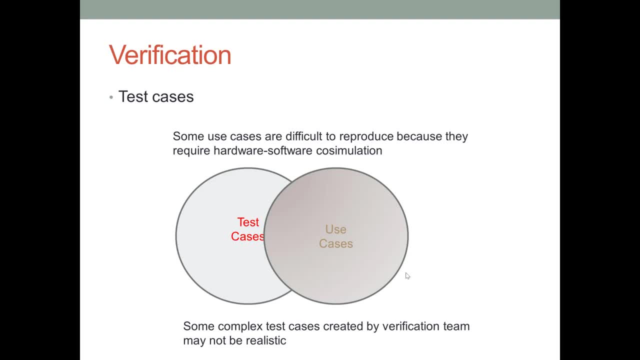 But if you have something here, Right, That means you verified something here And you have a set of all the actual use cases, Right. So you verified something here, But that was not even a use case, Right? It is a very peculiar test case that you created. 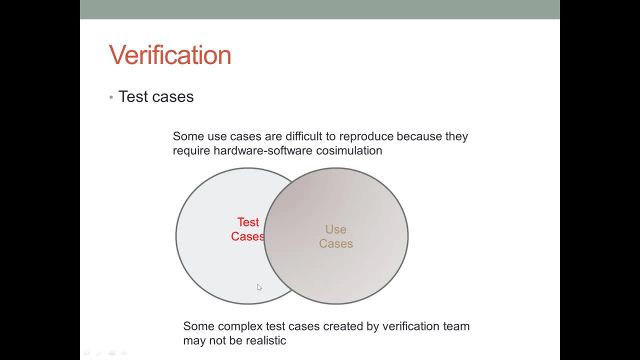 But in the practice that doesn't happen. So this may be a waste of the verification cycle time. Right On the other hand, this is even dangerous. So here is a situation where I have a use case But there is no corresponding test case there. 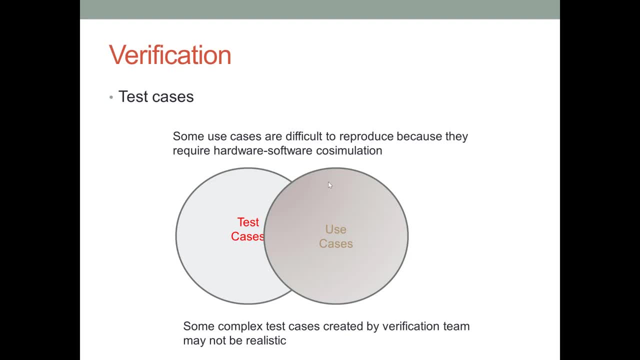 That means I never tested it for that particular situation Right. So both of these are not good Right. And because of the complexity of today's SOC, it is not easy to write these test cases Right. Sometimes you know if it is a very complex situation which requires you know something. 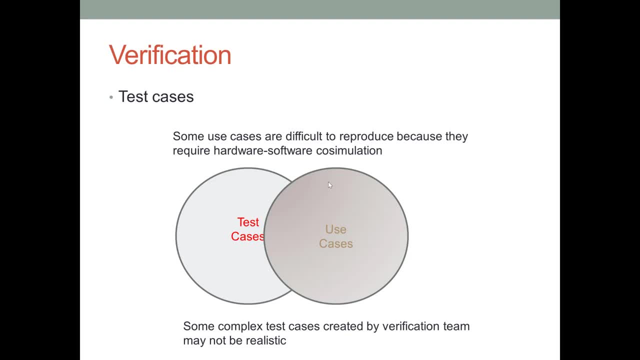 to happen in software And that software will generate a certain sequence of inputs- Inputs for the hardware and so on- Then the correct way is to do what is called as hardware software co-simulation Right, And so we have to be having a balance between creating unnecessary test cases which are 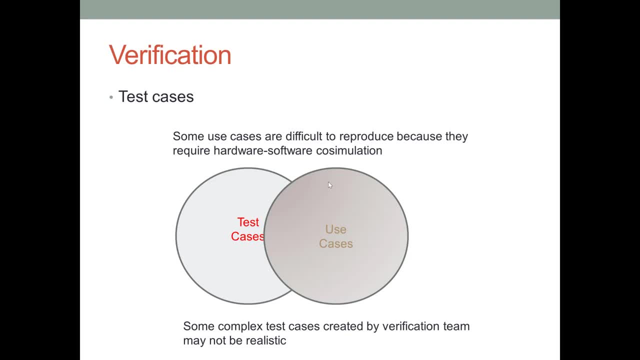 very complex Right And which are not realistic Versus missing out entirely on actual use cases. So this is where verification engineers have to play a very crucial role. So if you join a company as a verification engineer, you know you should try and maximize. 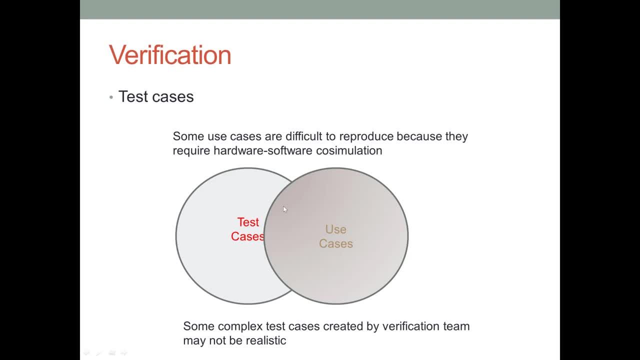 these kind of test cases. So if you create too many of these, you are really not contributing to the. you know better quality IP Right Or better quality of verification Right. So if you miss these, then definitely you are impacting and you are, you know, causing 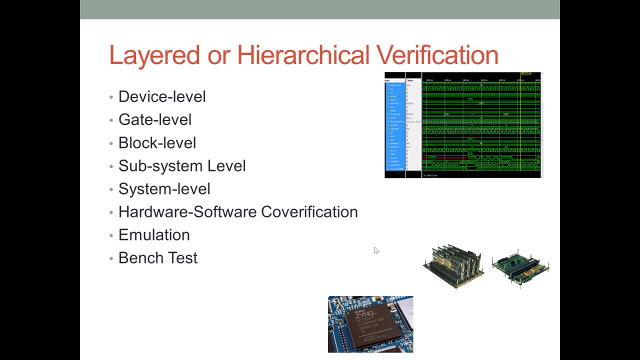 a risk, Right, All right, And verification has to happen at several different levels of abstraction. So if you are a person who is going to design small cells, Right, Maybe gates and stuff like that, Then you are performing mostly device level simulations by simulation. 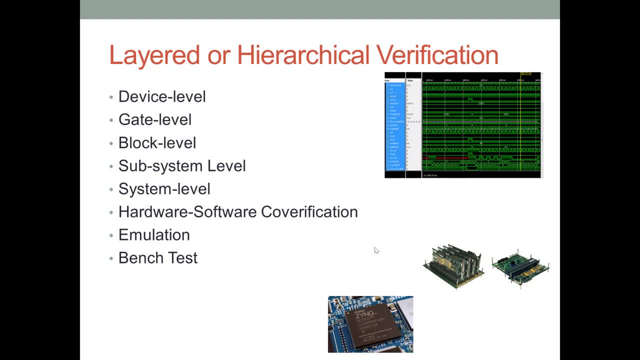 So that is one kind of verification that might happen. The other one is at the gate level. But gate level simulation is very expensive. Right, You cannot really do a gate level simulation of an SOC today, So people try to do it at a higher level of abstraction. 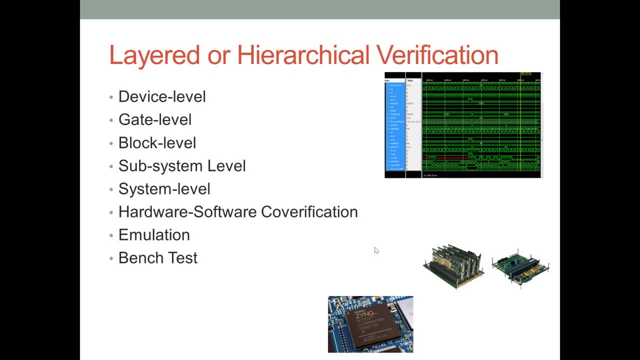 Right, You may have heard about system level simulation, system level design, So system Verilog is more and more popular today than Verilog itself. Right, Because system Verilog was sort of created with the assumption or with the sort of premise that more and more people are creating system on chip. 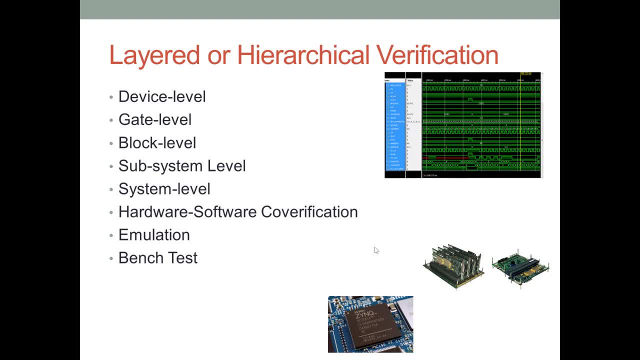 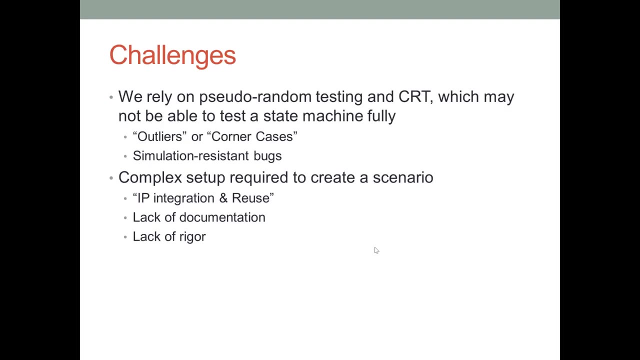 And it requires more complex tools for creating test benches. So creating test benches is a lot more easier with system Verilog than it is with, say, the you know Verilog or anything else Right? So what are some of the challenges, right, that people may face today? 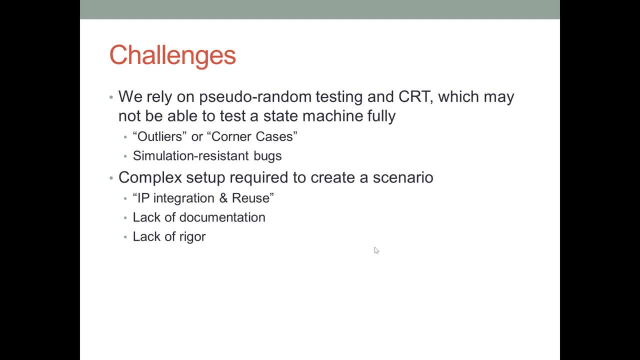 There are many Right, But you know a few of them are listed here. You know, if you are, if you have done system Verilog Right, You may be familiar with something called as constrained random testing. So random testing is a very common way we test IP. 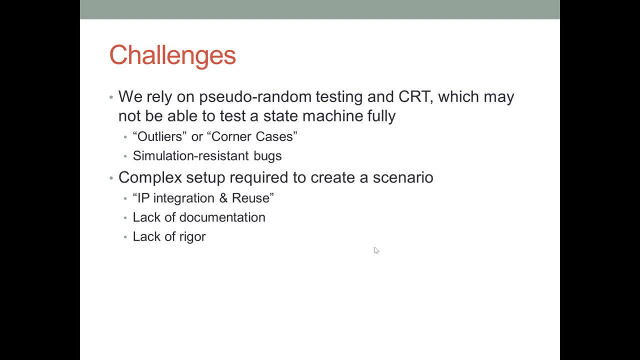 For example, I told you about the example of an addition Right. So there is a 32 bit adder Right. So since I cannot possibly generate all the 2 to the power 64 test cases, so what I can do is I can create a random sample of them. 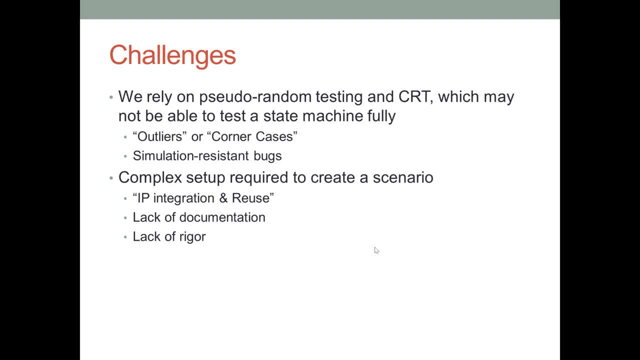 But when I do this, Okay, If I took, take it totally randomly, then you know, unfortunately I may miss out on very important ones like all 0.. Right, See, it is very important for the adder to handle 0 correctly, Right. 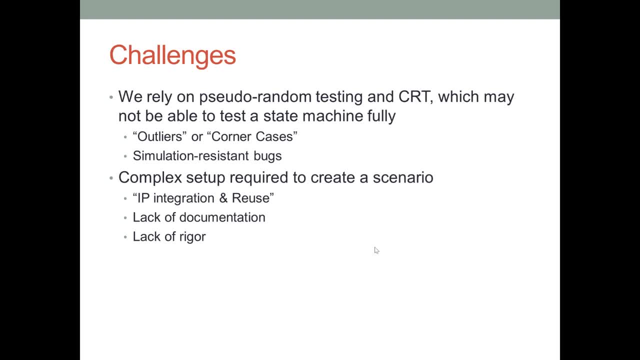 So 0 plus x is equal to x. Right, 0 plus 0 equal to 0. So these are very important test cases. So we may want to put certain constraints while generating the random test cases, saying that you know certain, the probability of certain bits you know being 1, or probability of a. 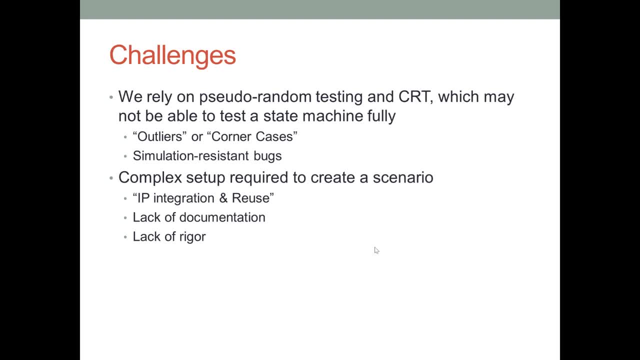 certain bit being 0. We may have to decide those up front, Right. So we tend to rely on pseudo random testing and constrained random testing. But you know we have to be aware that it may not entirely test a state machine fully, So there could be, you know, a deadlock situation or something like that which we could not. 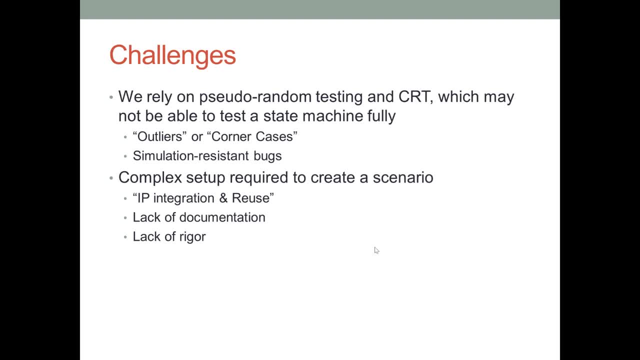 cover Right. So there may be a bug out there, which we call a simulation resistant, which means that it just does not get caught in simulation. We were never able to generate the test case Right And the other case could be. you know, the setup is very complicated. 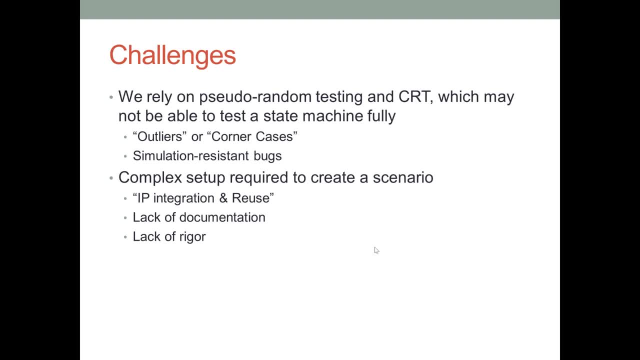 Right. To create that particular situation Right, A lot has to happen, A lot of activity, a lot of events have to occur before a particular event occurs in the system. So- and this is even more complicated because of IP integration and reuse- 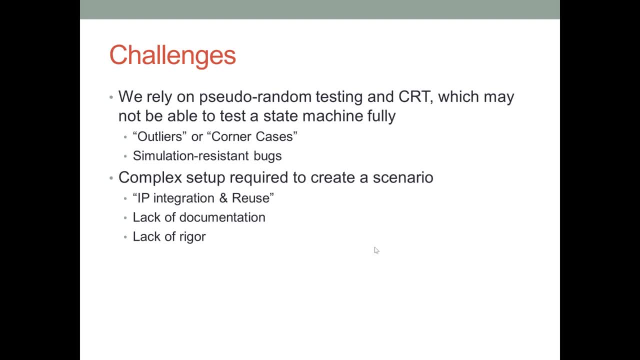 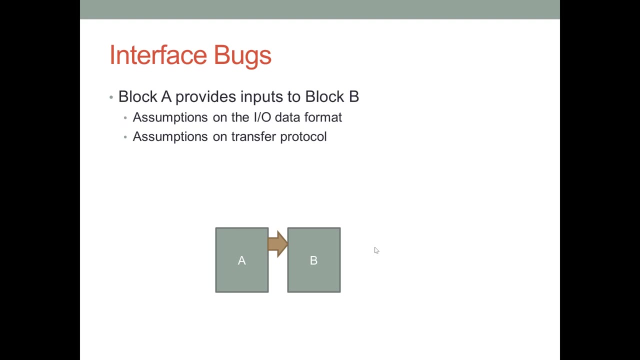 Right And because of the problems that I mentioned earlier: lack of documentation and lack of rigor in creating that IP on the documentation Right. So these are some of the difficulties, The bugs that can occur in the modern day ICs could be. I think I mentioned to you that. 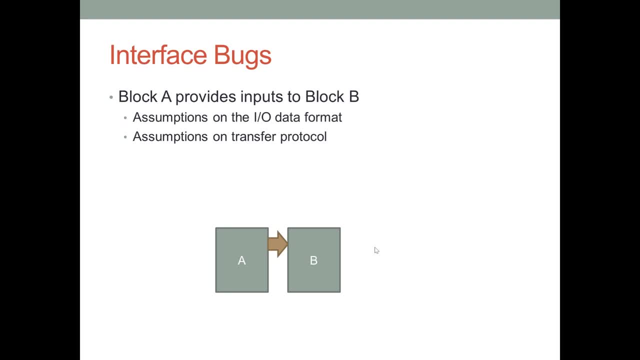 a person who integrates the IP, he may face interface challenges Right. So maybe there was not enough documentation to indicate Which is the most significant bit and which is the least significant bit, Or the fact that you know there is some sort of a encoding that has been done. 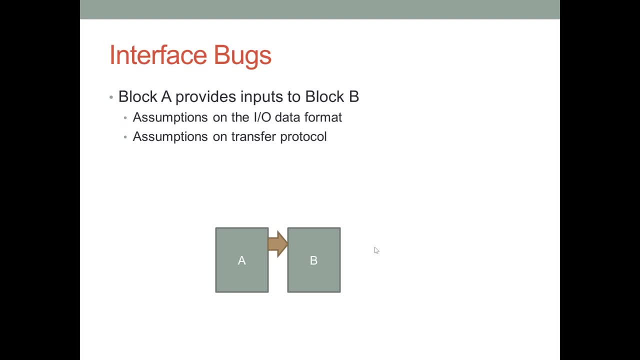 Right. So if these are not documented properly, there may be wrong assumptions made by the person who integrated the IP Right. The most significant bit may be connected to the least significant bit in the other block, Or let us say there is some sort of a error on the IP. 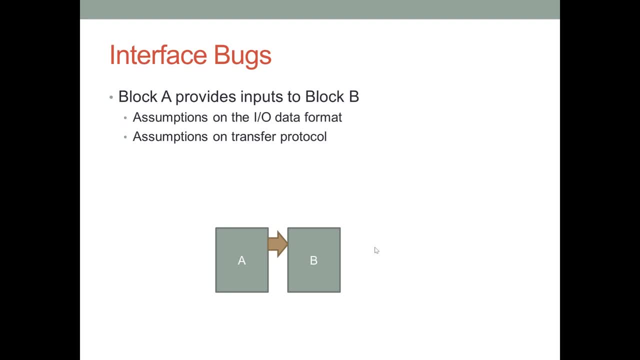 You may have heard about this multiple ways to represent, let us say, a block of data. Right, There are, you know, the big Indian and the little Indian methods. So the IPA may be providing a block of data in big Indian format and B may wrongly think. 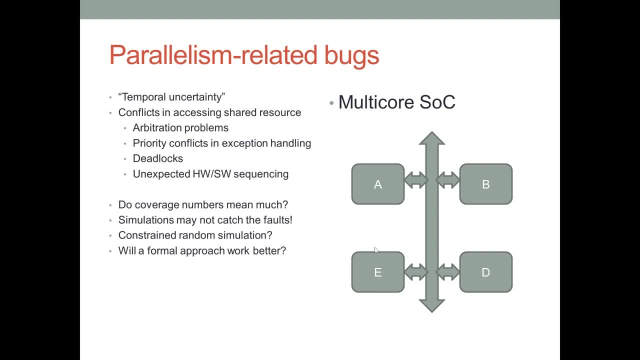 that it is little Indian. So these kind of bugs may exist. There may also be, You know, concurrency or parallel related bugs. See, concurrency can exist in today's chips. Right, You may have seen, Right, When you are using a cell phone, your cell phone has a lot of concurrency in it. 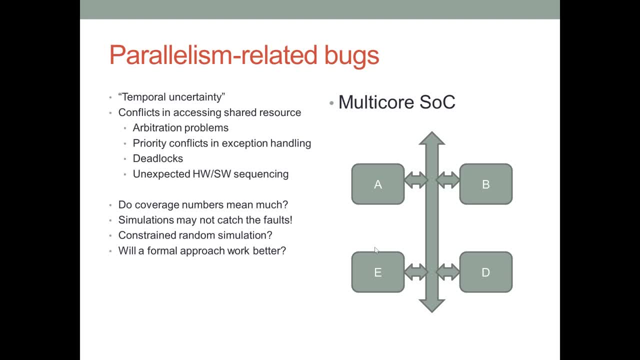 Right, It is simultaneously trying to, you know, maybe read some mails that you may have received. Also, you know it is parallel listening to any calls that may come in. There may be an SMS that may be received at the same time, or another app, maybe WhatsApp. 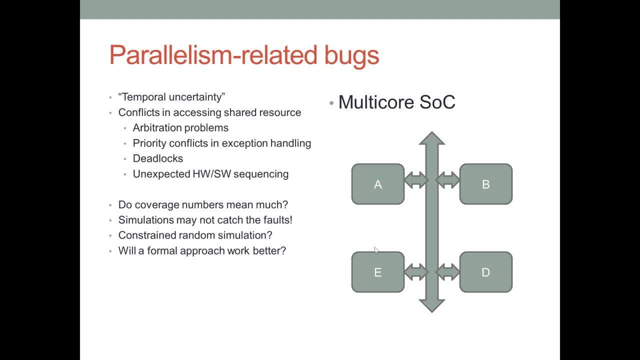 or something like that brings another. There is a lot of concurrency out there, Right? So you know. could there be a situation where you know something can go wrong and the system can get stuck somewhere? Maybe there is a you know deadlock that can occur and the system will never recover from. 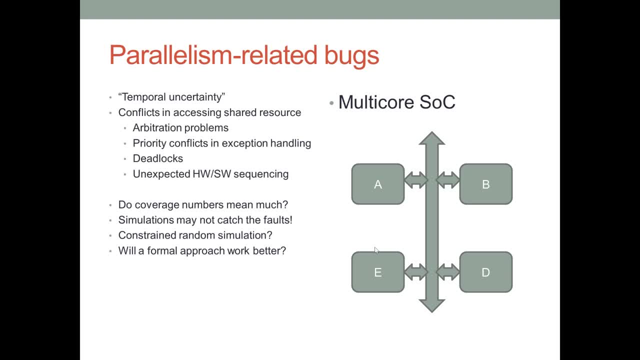 it. Or maybe there is a problem in arbitration. There are many resources that are being shared and maybe a situation occurs when a particular, you know task never gets serviced Right. Everybody else is being served, but this particular task is starved, It never gets a chance. 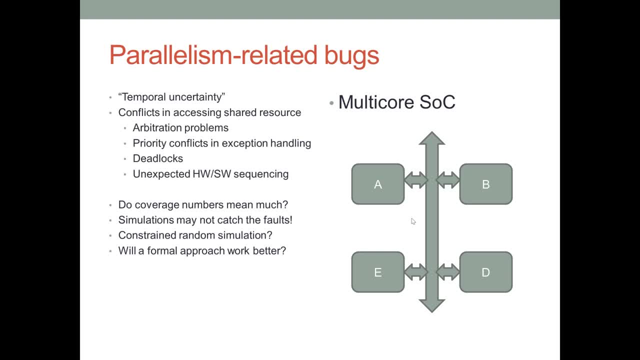 So these kind of bugs may exist, and to verify whether they exist or not requires a lot of thinking. You get a lot of you know: careful analysis, careful planning of the verification Right And, last but not the least, you know. you must be aware that you know, no matter how much. 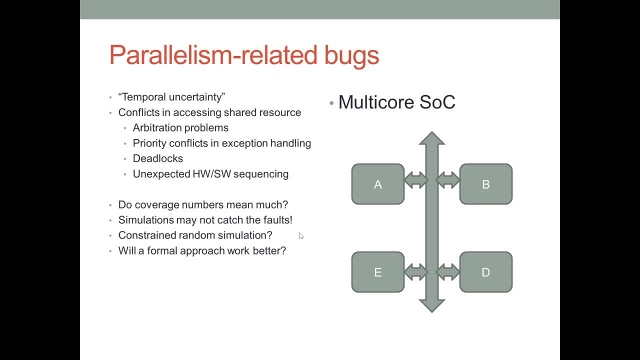 verification we do, Right, We cannot prove that the design has no functional bug. I hope everybody understood that There is a coverage concept, Right. We may say We had ten thousand lines of code in this verilog or system verilog file and I have. 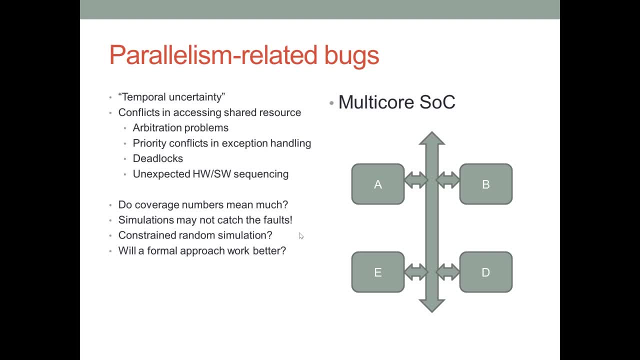 made sure that you know every one of them has been touched. Okay, But that may not mean much, Right? What if there are many? if then else, kind of branching When you touch that line which had the if then else. maybe you did not look at both the 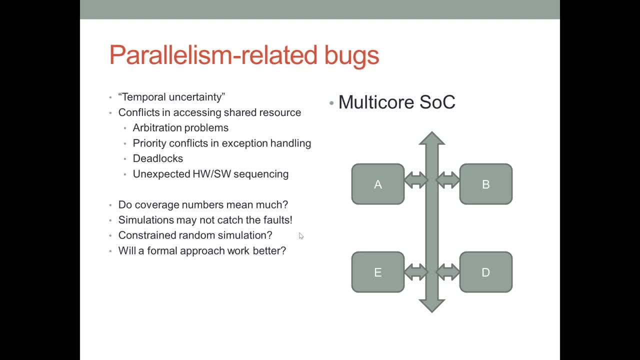 possibilities Right, And that will still count, for you know your coverage number. Similarly, simulations may not catch. you know all the faults Right, Because we may not have simulated all possible test cases And therefore you know we may have to look at alternate formal approaches as well. 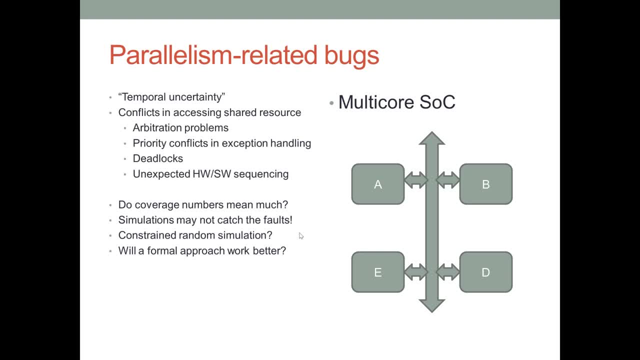 There are a lot of people who work on formal verification, where we can sort of try and prove that a design has no deadlock situation, or it has no starving kind of a situation, or there is no conflict that will cause a particular kind of a, you know, resource conflict. 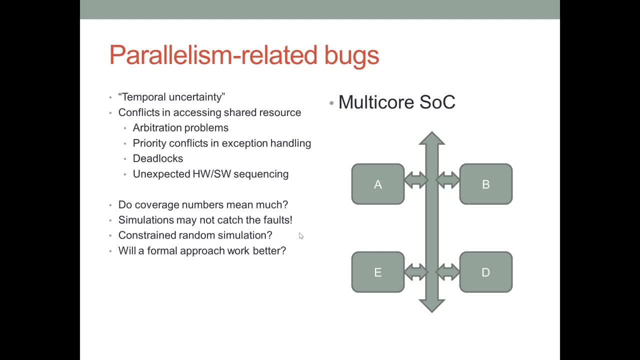 or something like that. So these are formal verification methods and people do work on formal verification. The constant complaint about formal verification is that it tends to be very competition intensely for large designs So they are not able to do it for large designs, They are only able to do it at small block level. 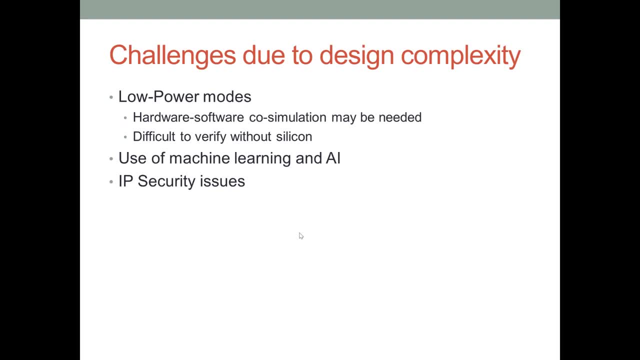 Right. And there are other challenges. for example, today the IPs may have many modes of operations, such as low power modes of operation, And you know we may require some hardware, software co-simulation in order to verify all these low power modes Right, And sometimes without silicon. you know the verification is very, very difficult. 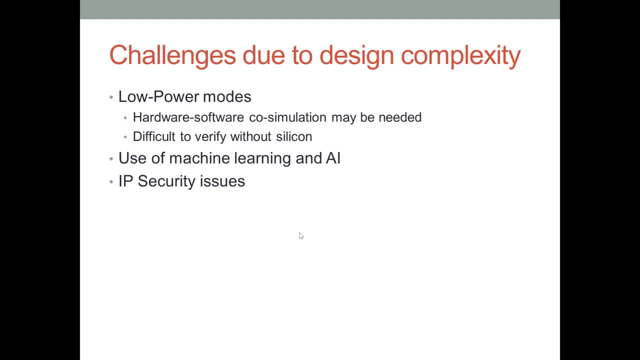 And slowly. people are trying to ask the question whether we can use things like machine learning and artificial intelligence to be able to select better quality tests Right, And to improve, you know, the verification process. Plus, there are other issues like IP security. What if the IP is doing something that? 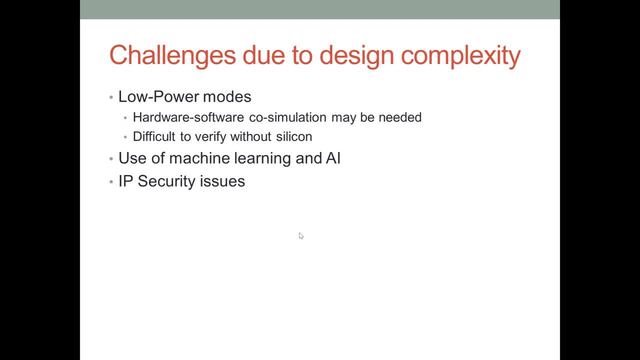 Is more than its functionality. Right, Maybe it has a security bug, Maybe what we call as a untrustworthy IP. It may do something dangerous. Right, It may be communicating to the outside world some data that is not expected to be communicated.